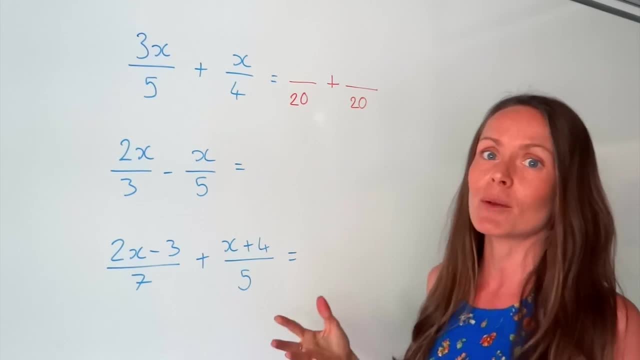 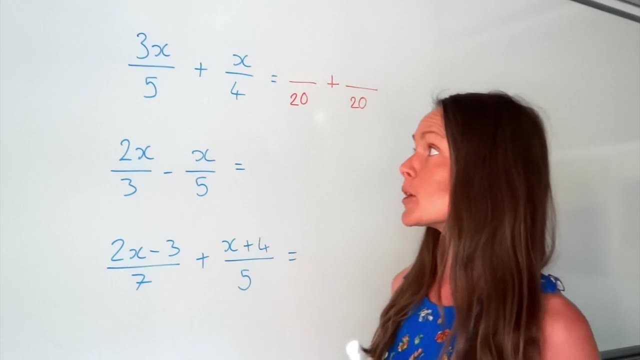 could choose a bigger number. but it's good if you choose a smaller number because it means less simplifying Later on in the question. So you can't just go changing the denominator, because you need to find what we call an equivalent fraction. So if you change the denominator you must. 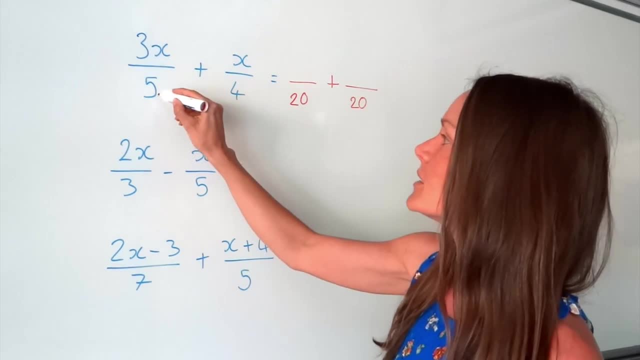 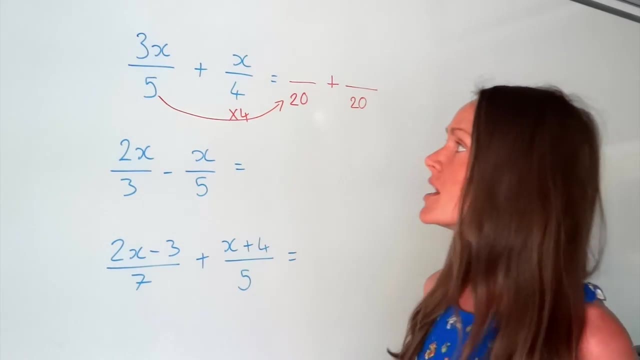 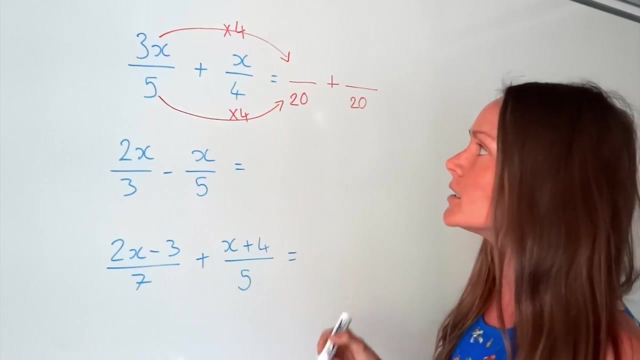 change the numerator as well, so the number on top. So if we take the first fraction to change from 5 to 20, well, I multiplied that number 5 by 4.. So I have to do exactly the same thing with the numerator. So I have to multiply that 3x by 4 as well, So 3x multiplied. 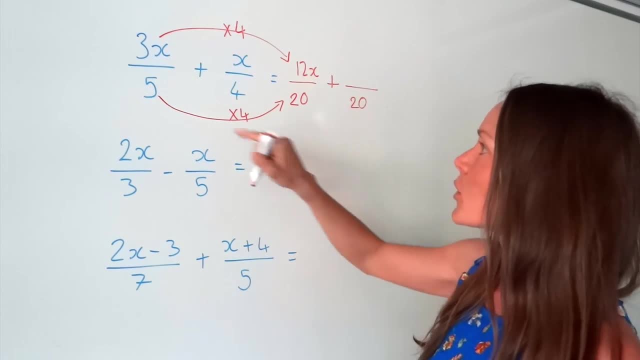 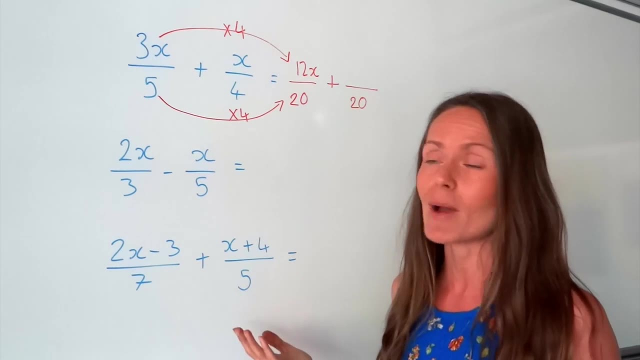 by 4 gives me 12x. So this is exactly the same fraction as this one. they're called equivalent fractions. We're just writing them in a different format so that we're allowed to add them later on. So let's look at the next one. 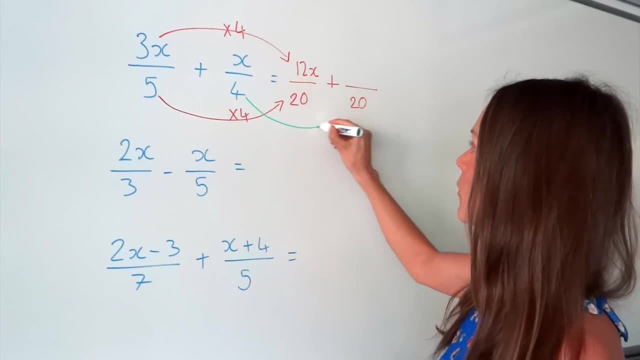 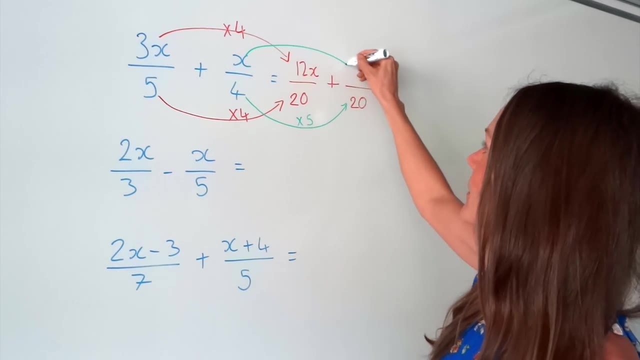 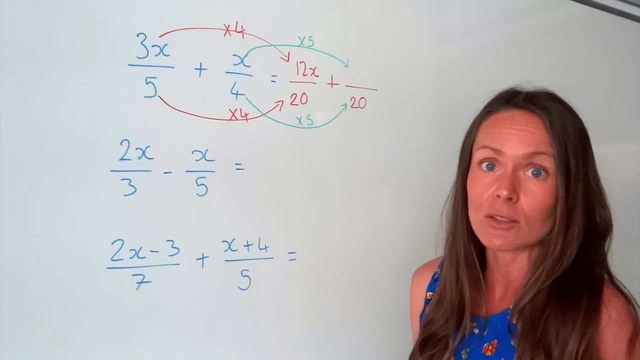 So in the next example we were changing 4 to 20. So this time we multiplied that number by 5.. So again you have to do exactly the same thing with the numerator and multiply that by 5. as well. So x multiplied by 5 is just 5x, Now that I've got the common denominators. 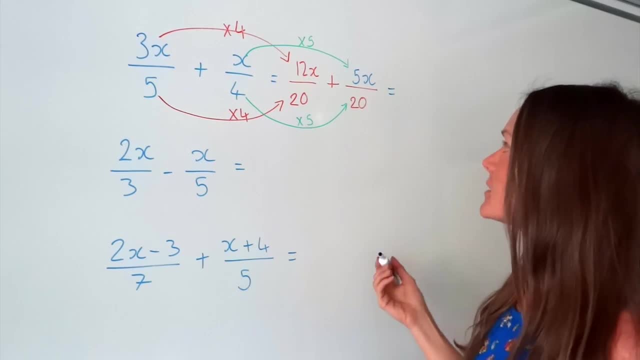 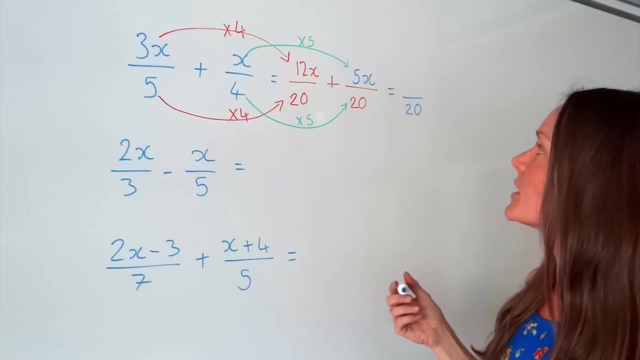 I'm allowed to add the two fractions together. Remember, when you're adding or subtracting, the denominator doesn't change, So this one is still the same, But the top two numbers here we can add them together And we can actually add these and simplify these two terms, Because 12x. 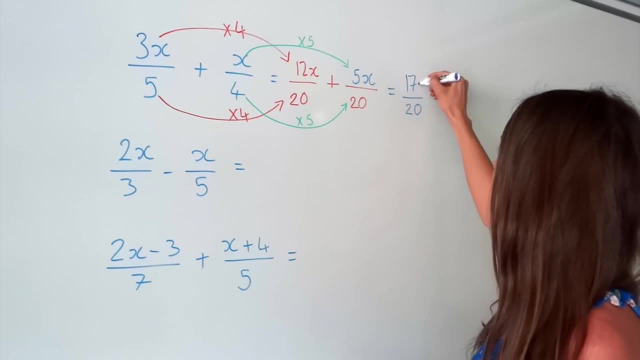 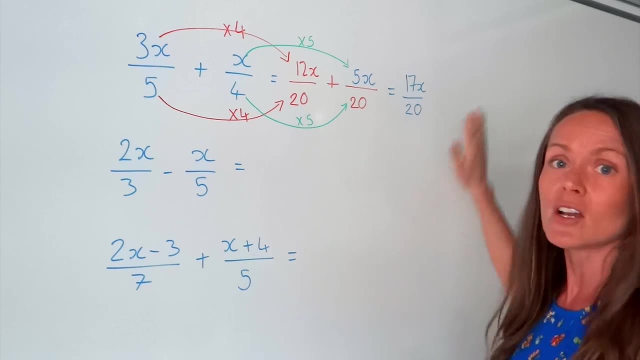 plus 5x is 17x, And that's my final answer. I can't simplify this fraction because there's no common factor in 17 and 20.. So I'm done with that one. Now on to the next one. Again, you need to. 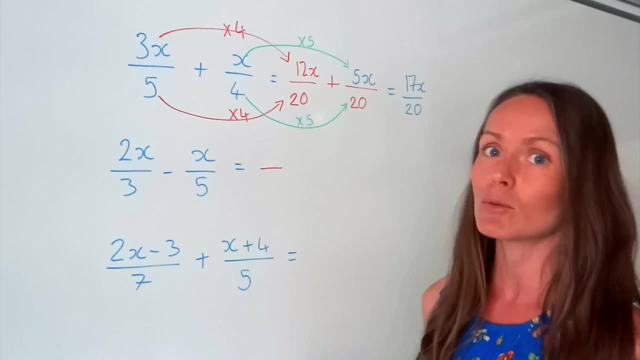 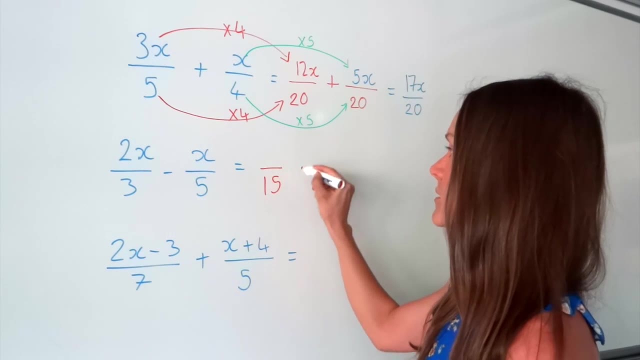 find a common denominator. So the lowest common multiple of 3 and 5, so the smallest number that both 3 and 5 fit exactly into is 15.. So remember, it's the same throughout, even at the end, because it's the lowest common number. So it's the lowest common number, So it's the lowest. 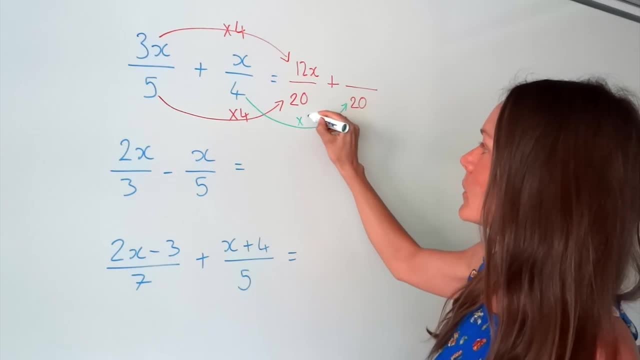 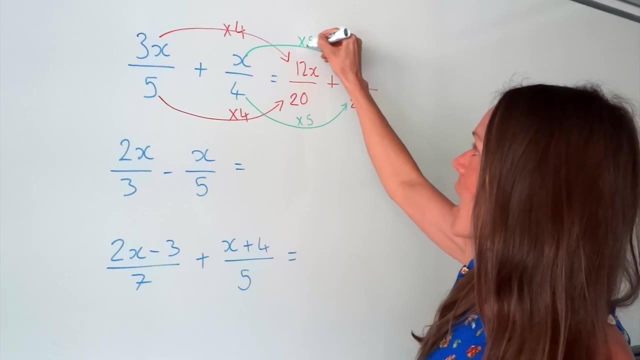 changing 4 to 20.. So this time we multiplied that number by 5.. So again, you have to do exactly the same thing with the numerator and multiply that by 5.. So this is exactly the same thing with the numerator, and multiply that by 5 as well. So x multiplied by 5 is: 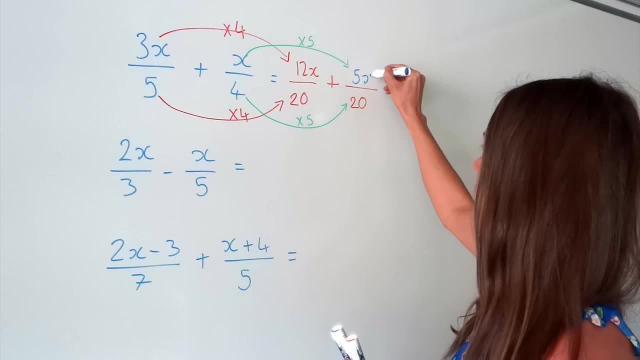 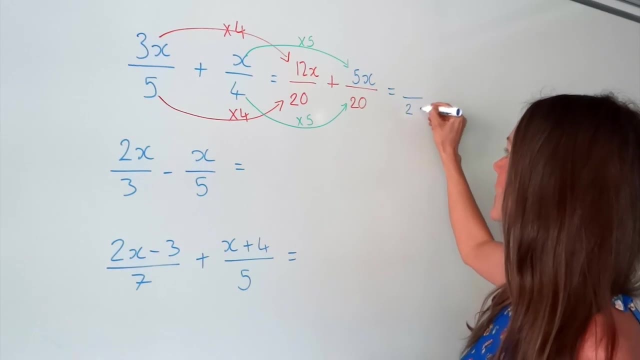 just 5x. Now that I've got the common denominators, I'm allowed to add the two fractions together. Remember, when you're adding or subtracting, the denominator doesn't change. So this one is still the same. But the top two numbers here. we can add them together And we can. 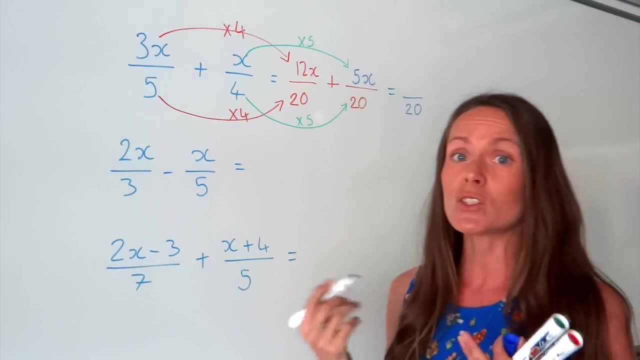 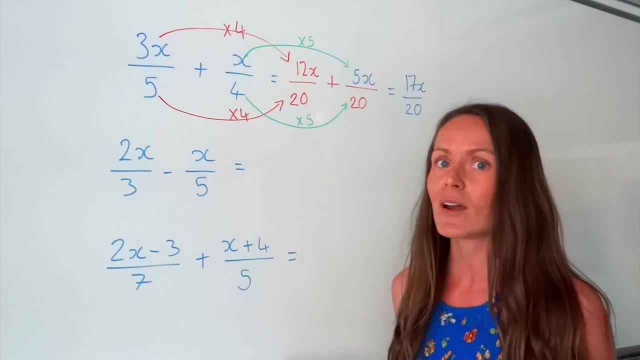 actually add these and simplify these two terms, Because 12x plus 5x is 17x, And that's my final answer. I can't simplify this fraction because there's no common factor in 17 and 20.. So I'm done. 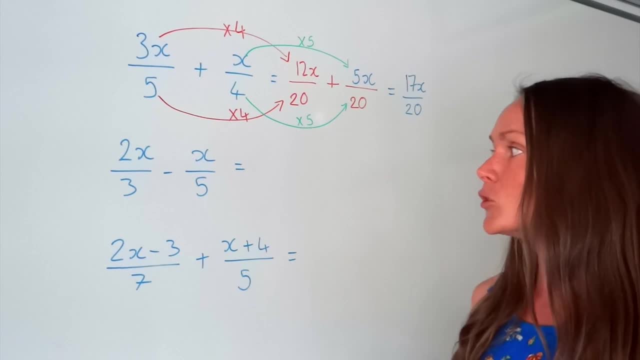 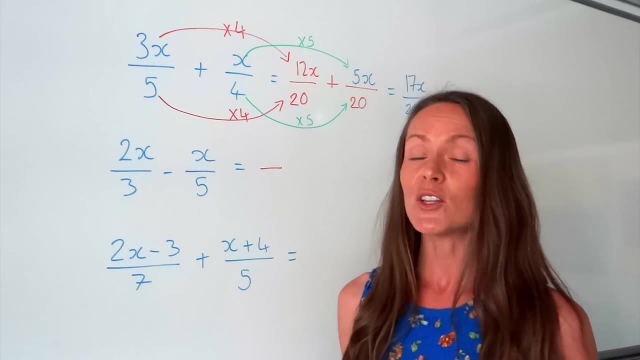 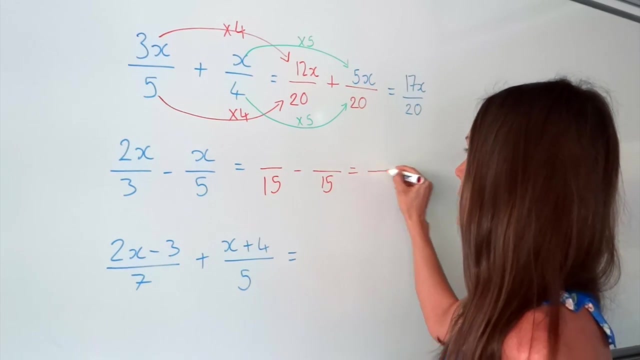 with that one. Now on to the next one. Again, you need to find a common denominator. So the lowest common multiple of 3 and 5, so the smallest number that both 3 and 5 fit exactly into is 15.. So remember, it's the same throughout, even at the end, because 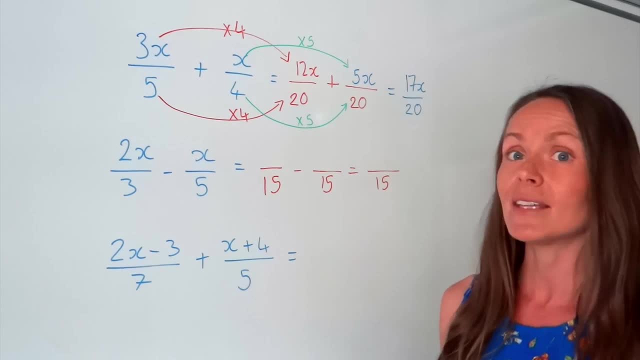 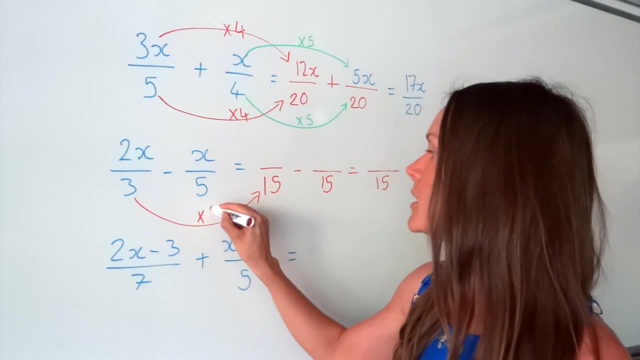 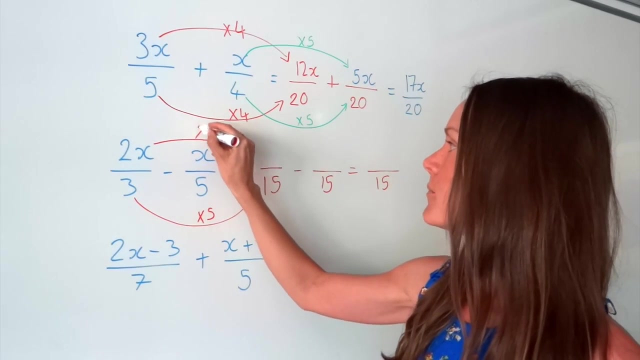 the denominator doesn't change, But now we need to find the equivalent fractions. So you can't just go changing 3 to 15. You have to change the numerator as well. So to get from 3 to 15, I have to multiply by 5. So I do the same with that numerator. there I 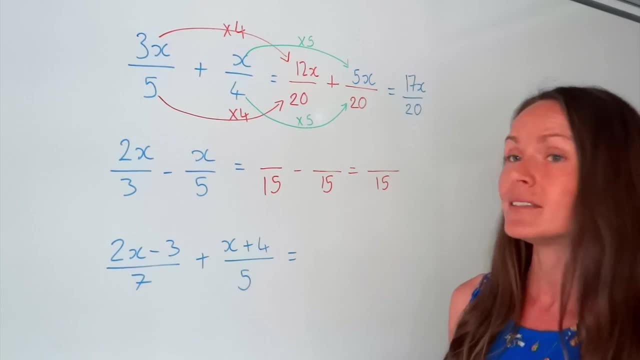 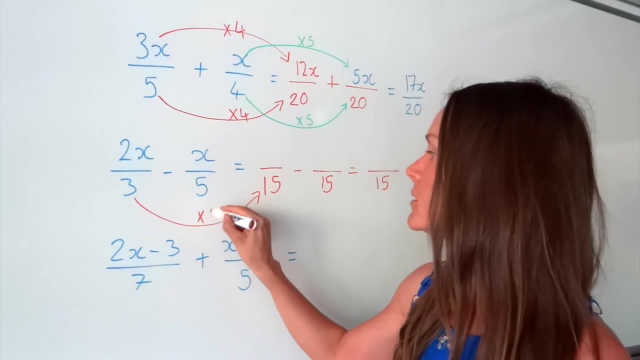 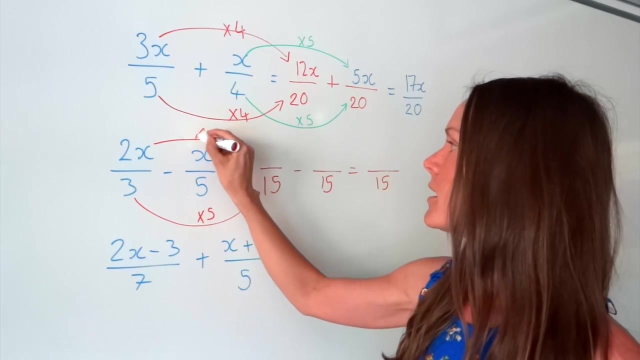 common number because the denominator doesn't change. But now we need to find the equivalent fractions Because you can't just go changing 3 to 15. You have to change the numerator as well. So to get from 3 to 15, I have to multiply by 5. So I do the same with that numerator there. 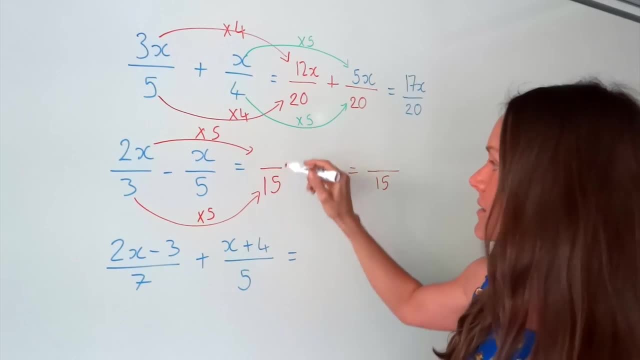 I multiply by 5.. So 2x times 5 is 10x. And then I do the same with the second fraction. So to get from 5 to 15, I times by 3.. So I do the same with the second fraction. 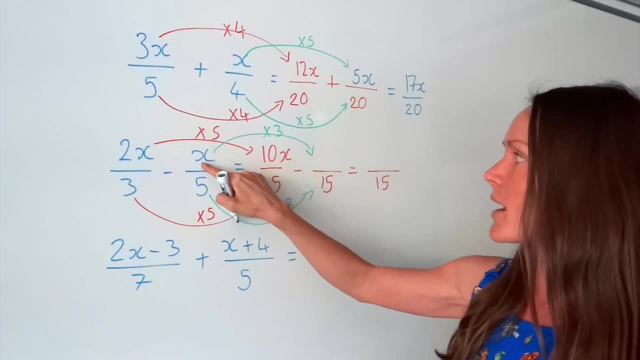 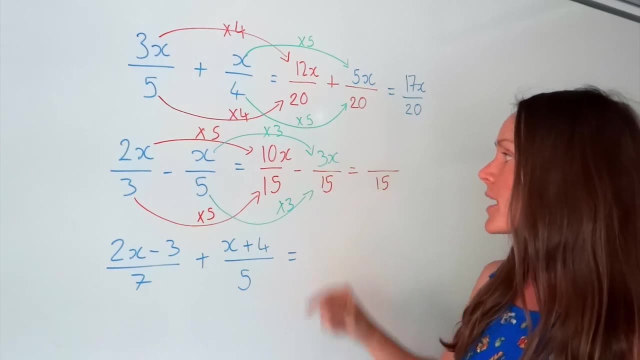 So I do exactly the same thing with the numerator. So x times 3 is 3x. Watch out this time, because we're subtracting. So 10x, take away 3x leaves me with 7x, And again, I can't simplify this answer. 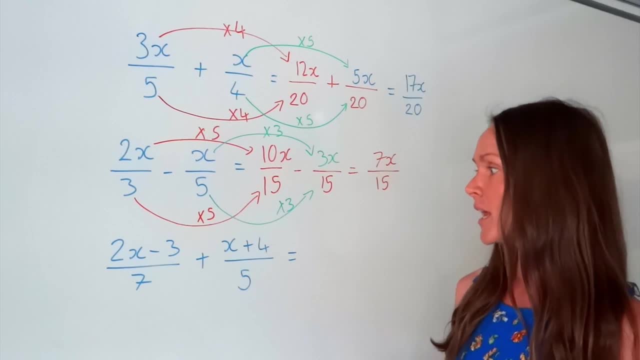 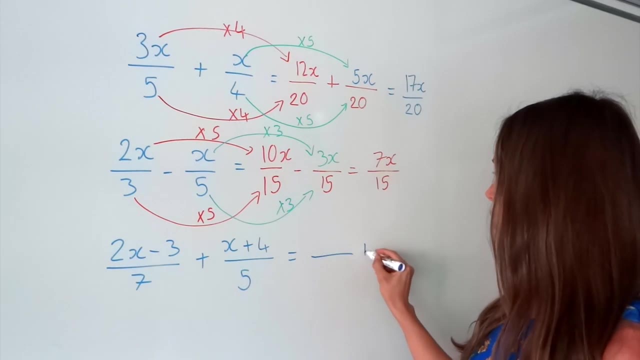 because there isn't a common factor in 7 and 15.. Now on to the last one. Okay, I'll do some hard ones afterwards, but just for now. So again, the lowest common multiple, so the smallest number that both 7 and 5 fit exactly into, is 15.. So I do the same with the numerator. So x times 3 is 3x, And 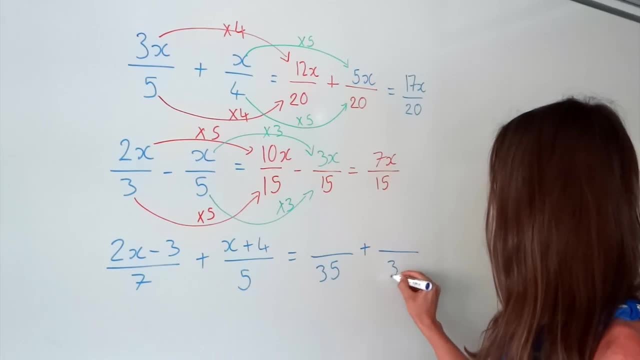 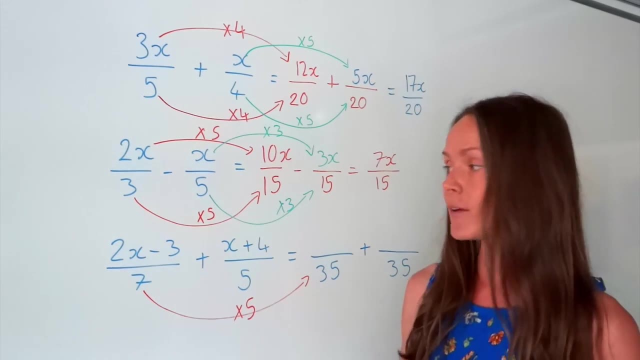 again the lowest common multiple. so the smallest number that both 7 and 5 fit into is 35. So do that bit first. Now, to get from 7 to 35, I must multiply by 5. So I have to do the same with all of this. 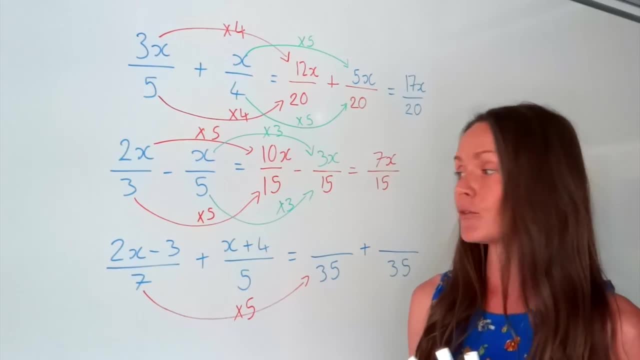 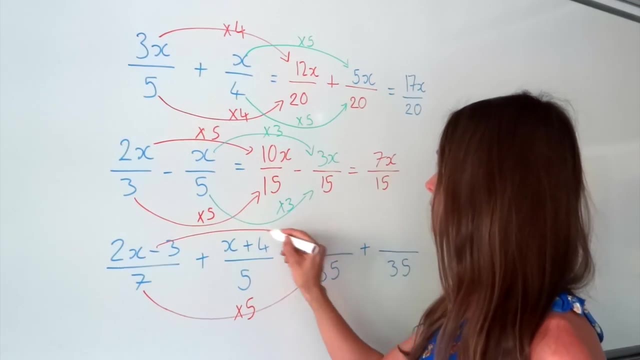 I have to multiply this entire numerator by 5.. So here we only had one term, but now we've got two things we have to multiply by 5.. So if I multiply 2x by 5, I get 10x. 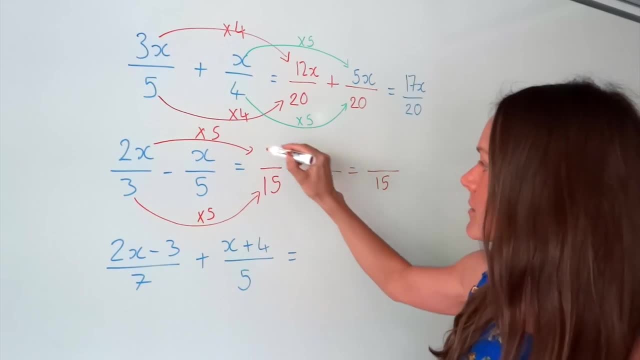 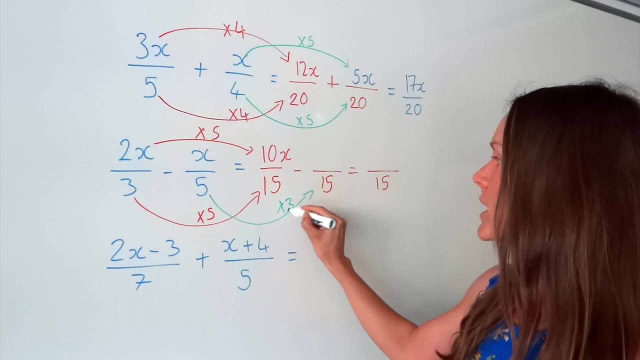 multiply by 5.. So 2x times 5 is 10x. And then I do the same with the second fraction. So to get from 5 to 15, I times by 3.. So I do exactly the same thing with the numerator. 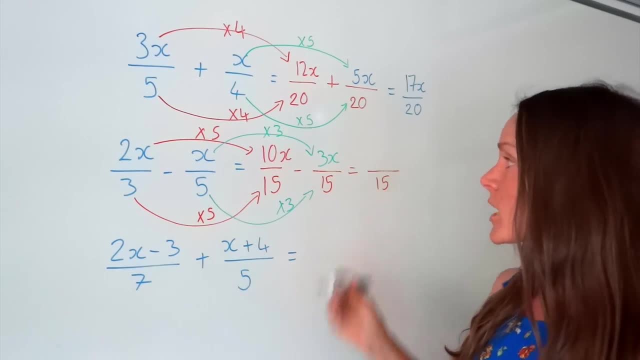 So x times 3 is 3x. Watch out this time because we're subtracting. So 10x, take away 3x leaves me with 7x. And again, I can't simplify this answer because there isn't a common factor in 7 and 15.. 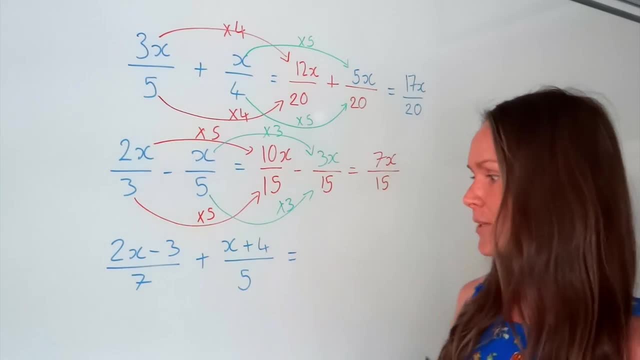 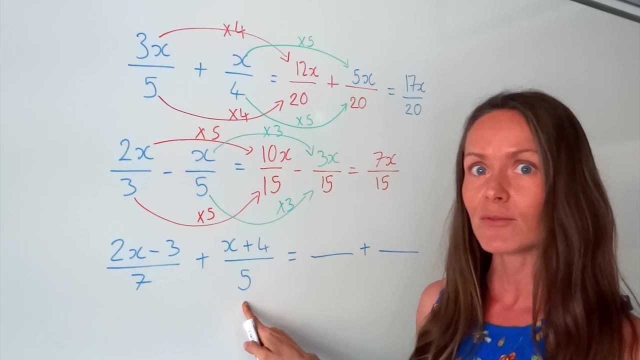 Now on to the last one. OK, I'll do some hard ones afterwards, but just for now. So again the lowest common multiple, so the smallest number that both 7 and 5 fit into is 35.. So do that bit first. 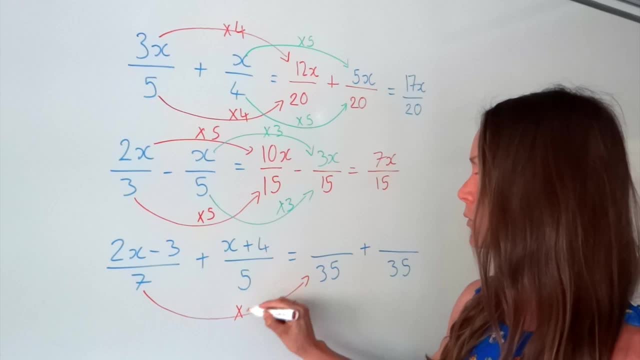 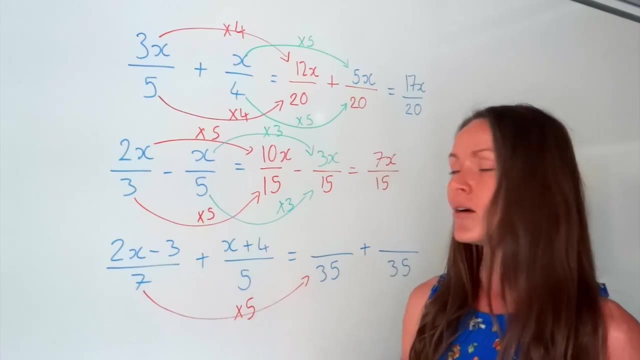 Now, to get from 7 to 35, I must multiply by 5.. So I have to do the same with all of this. I have to multiply this entire numerator by 5.. So here we only had one term, but now we've. 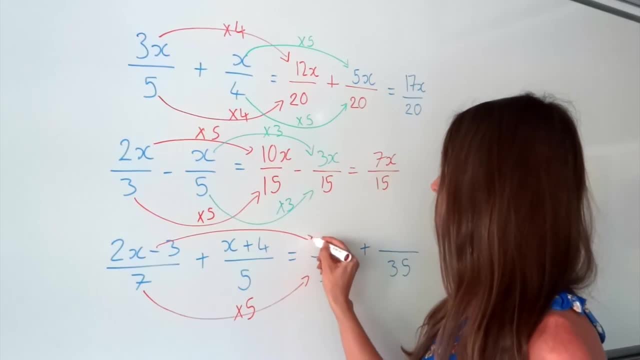 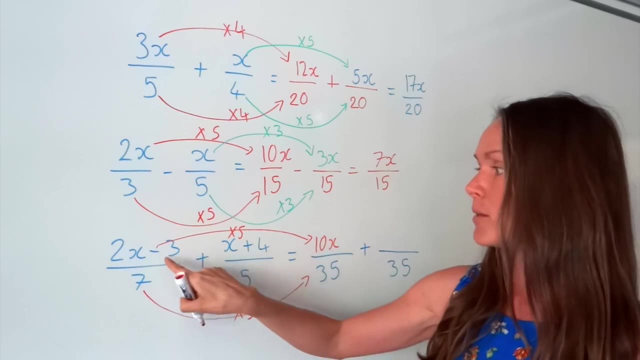 got two things: we have to multiply by 5.. So if I multiply 2x by 5, I get 10x, And if I multiply negative 3 by 5, I get negative 15. So we've got 2x. 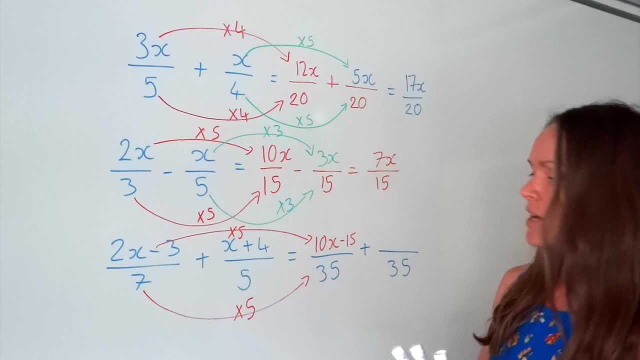 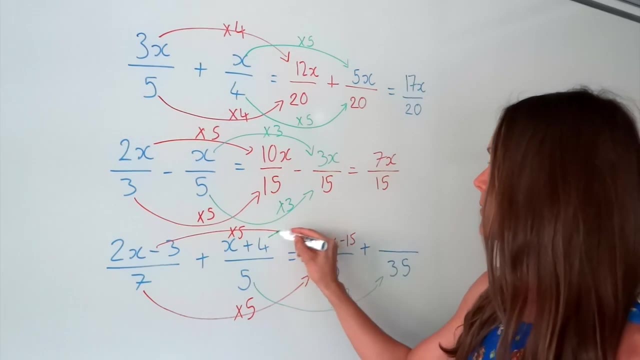 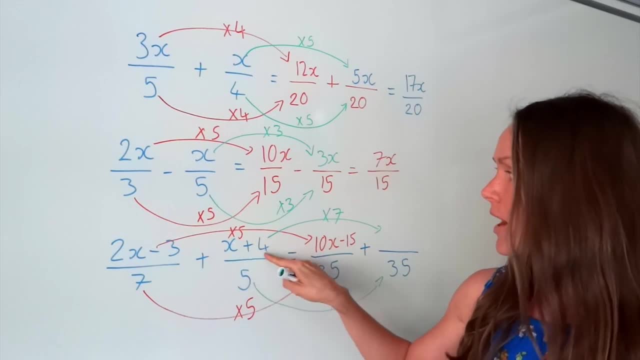 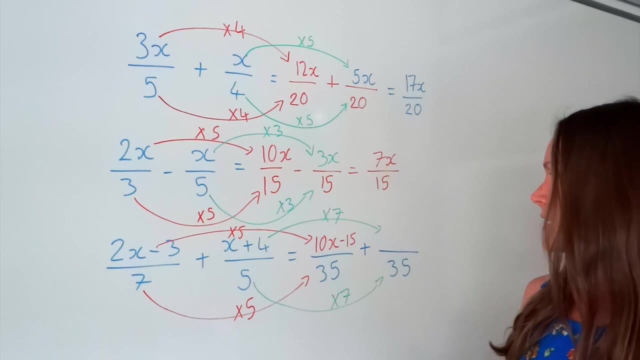 And again, watch out, because there are two terms here that I have to multiply by 7.. So we've got x multiplied by 7,, which is 7x, And we've got 4 multiplied by 7, which is positive 28.. So right, plus. 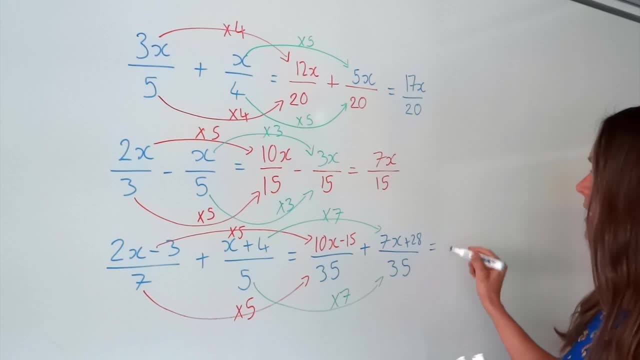 And now we can add them together. So we're still not finished. Now that we've got the common denominator, we can add them together. Remember, the denominator stays the same. We're adding the terms together. So 10x plus 7x gives me 17x, And the numbers be careful. 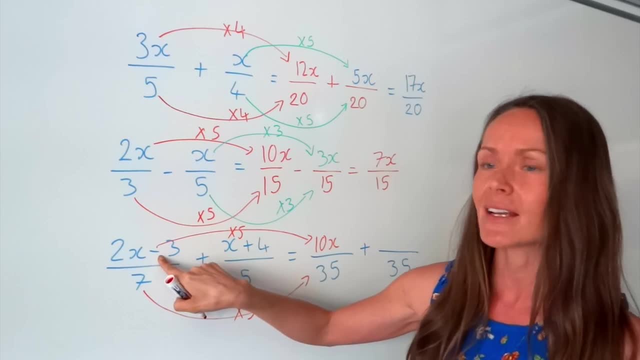 And if I multiply 2x by 5, I get 10x. And if I multiply 2x by 5, I get 10x. And if I multiply negative 3 by 5, I get negative 15.. So we've got two things we have to write on. 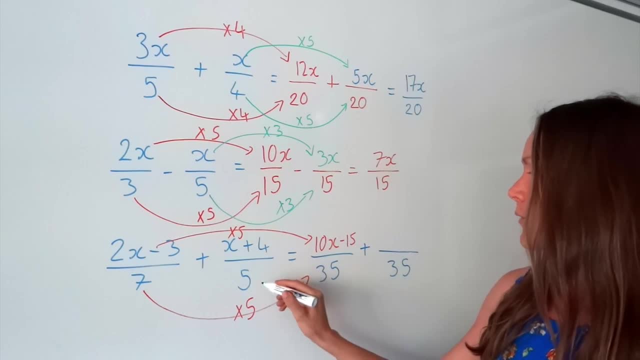 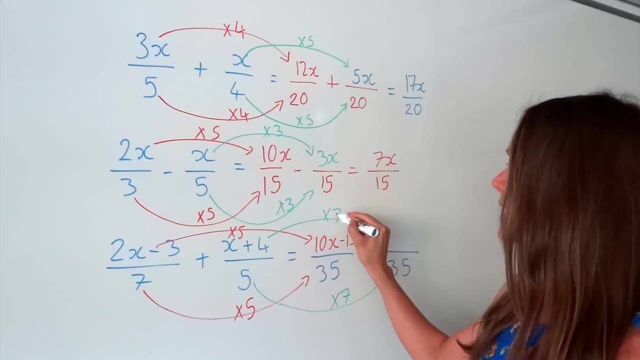 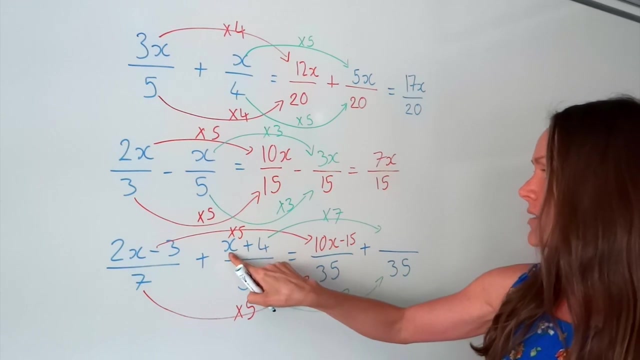 this numerator here. So for the second fraction to get from 5 to 35, I must multiply by 7.. So I do the same thing with the numerator And again, watch out, because there are two terms here that I have to multiply by 7.. So we've got x multiplied by 7, which is 7x. 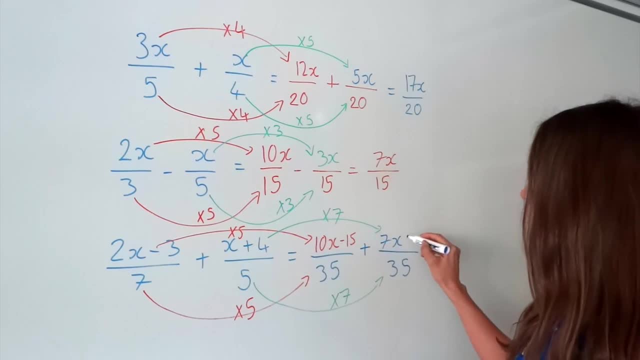 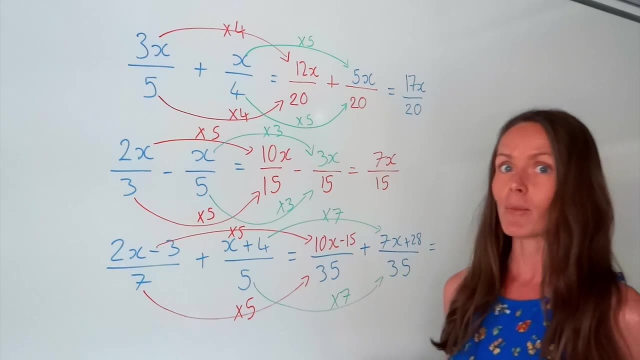 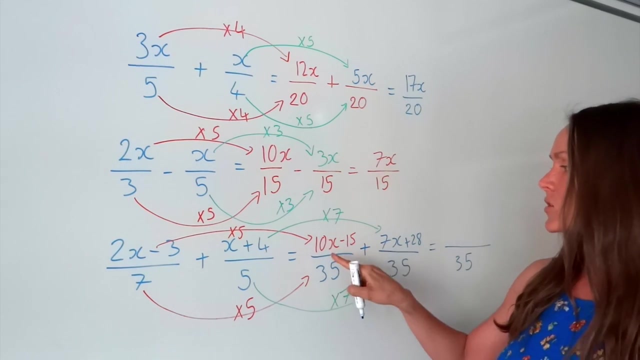 And we've got 4 multiplied by 7, which is positive 28.. So I write plus And now we can add them together. So we're still not finished. Now that we've got the common denominator, we can add them together. Remember, the denominator stays the same. We're adding the terms together, So 10x. 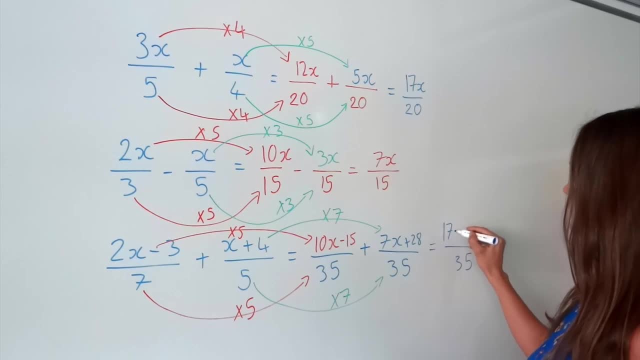 plus 7x gives me 17x, And the numbers be careful, because this one's negative. We've got negative. 15 plus 28, which gives me 17x, And the numbers be careful, because this one's negative, We've got. 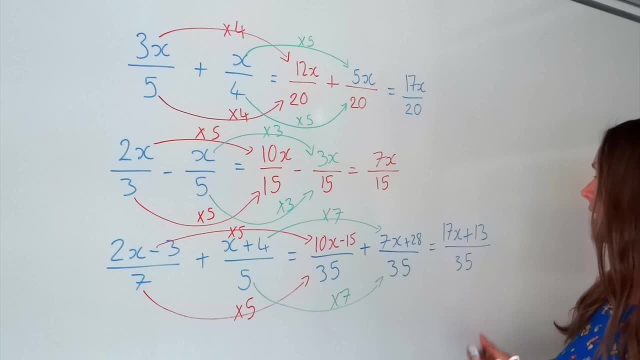 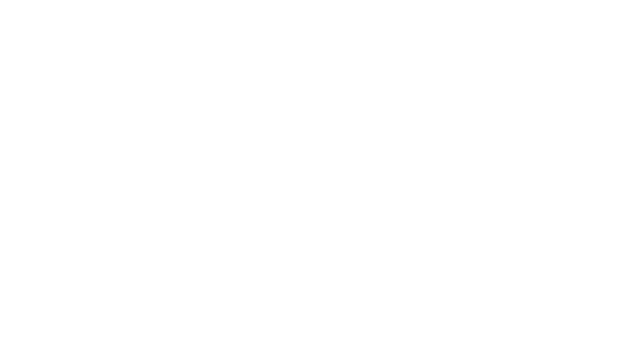 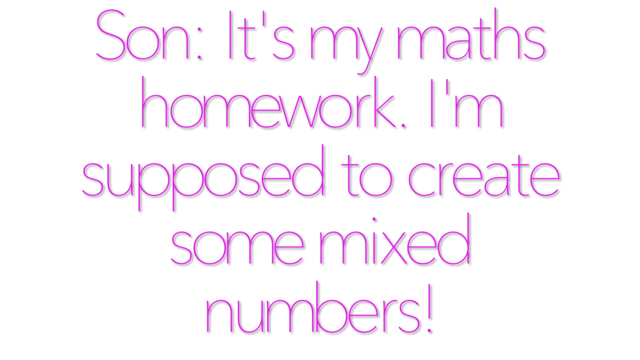 negative: 15 plus 28,, which gives me 13x. And just like the other two, this one doesn't simplify because there isn't a common factor within these numbers. All right, I'm going to keep making them harder. Okay, so, just like before, I need to start by finding the common denominator, which is 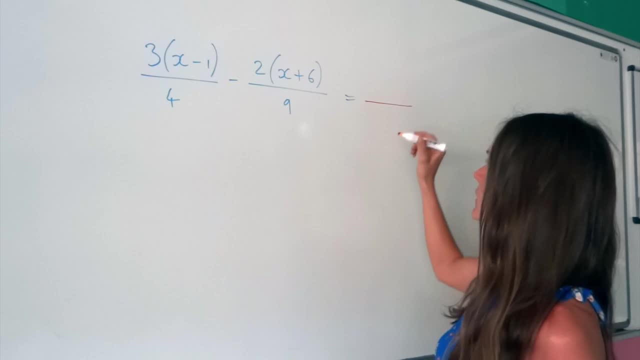 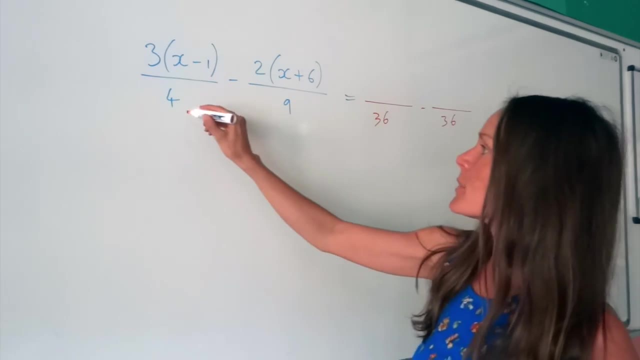 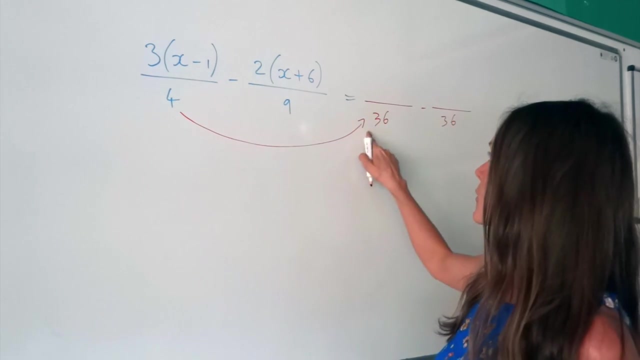 for these two fractions. So the smallest number that both 4 and 9 fit into is 36.. So I found my common denominator, But remember, we need to change the numerators as well to find the equivalent fractions. So to change 4 to 36, I have to multiply that number by 9.. So I do the same with: 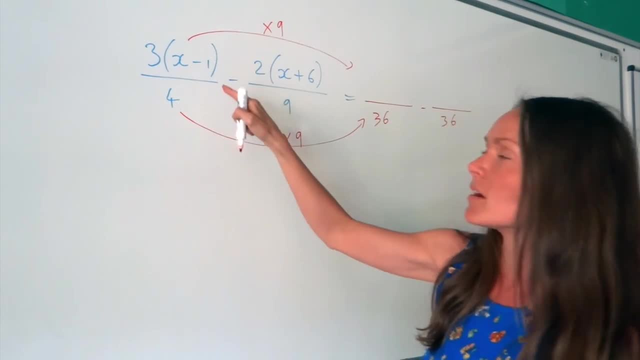 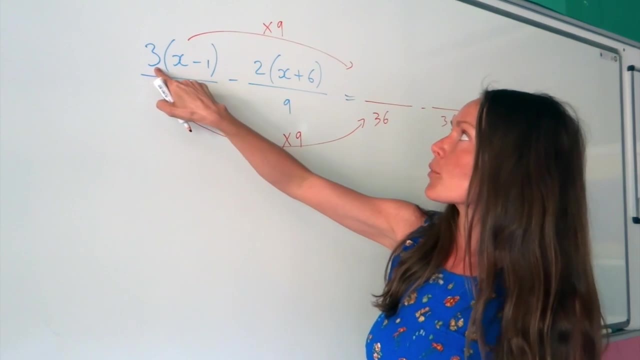 the numerator And I multiply this numerator by 9.. Well, when I multiply this by 9,, I'm going to multiply this numerator by 9.. So 3 times 9 is 27.. And this bracket? I can just leave that there for. 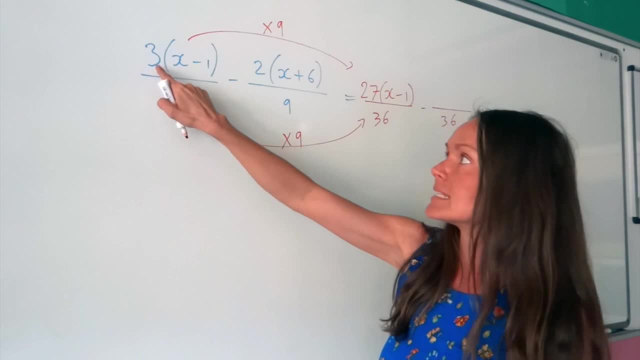 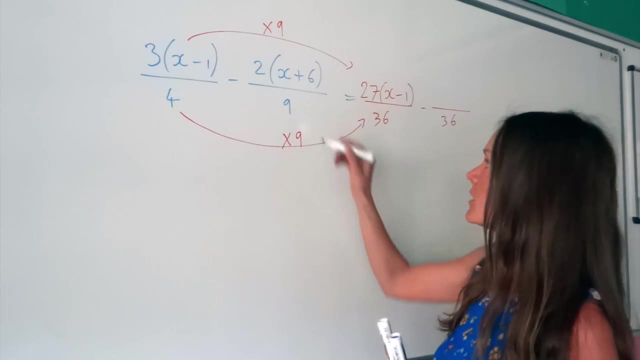 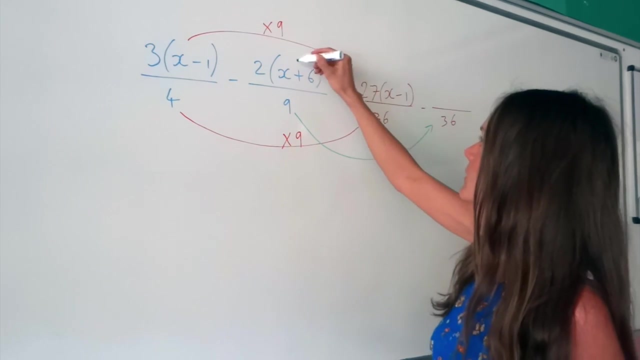 the moment. Okay, so multiplying this number by 9 is the same thing as multiplying this whole numerator by 9.. And I'm going to do exactly the same thing with the second fraction, except this time, to get from 9 to 36,, we must multiply by 4.. So I'm going to do the same with this numerator. 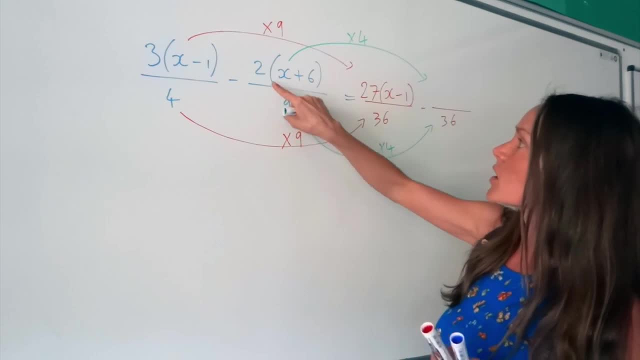 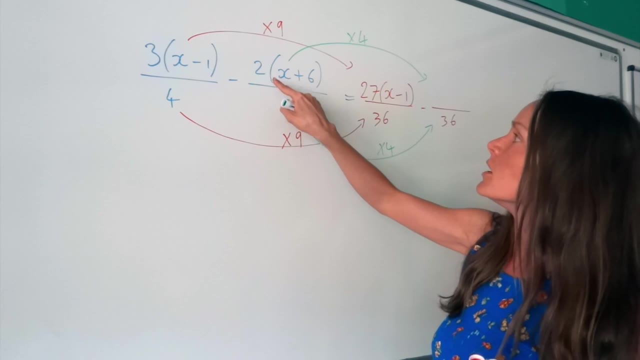 and I'm going to multiply by 4.. So, just like before, you only need to multiply this number by 4.. It's the same thing as multiplying the whole thing by 4.. So 2 multiplied by 4 is 8. And the bracket just stays the same. 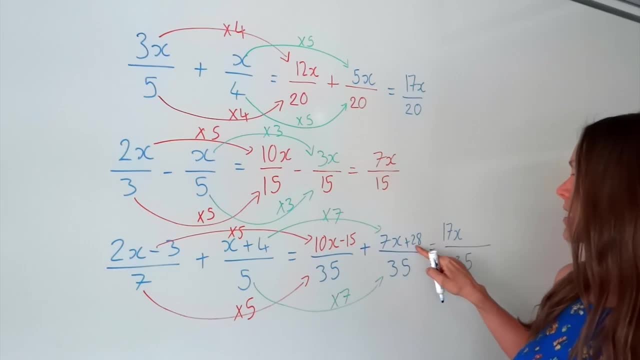 because this one's negative. We've got negative 15 plus 28,, which gives me 13.. And, just like the other two, this one doesn't add up. So we've got negative 15 plus 28,, which gives me 13.. And this one doesn't simplify because there isn't a common factor within these numbers. 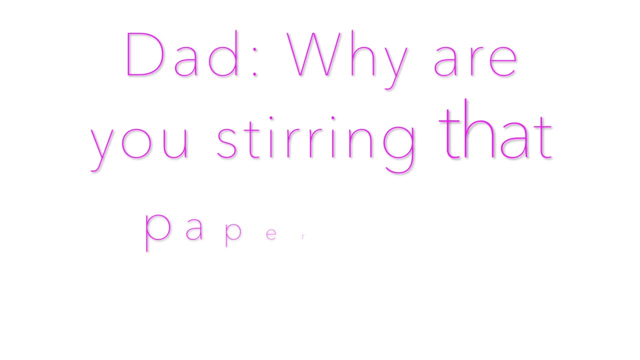 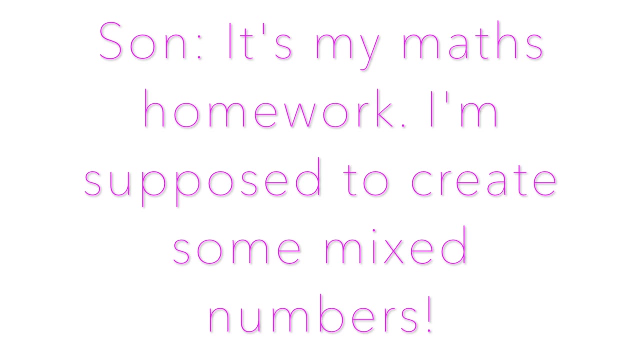 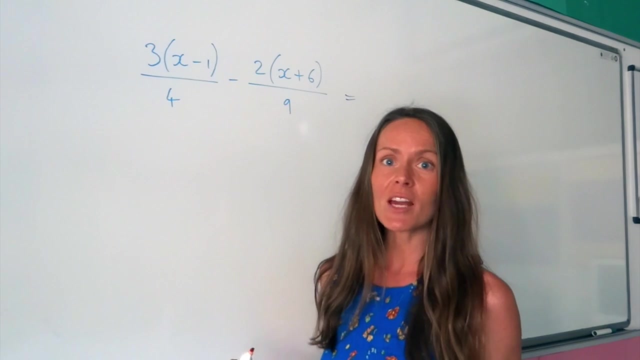 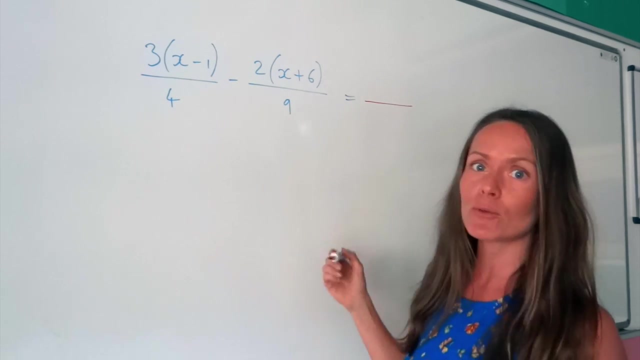 All right, I'm going to keep making them harder. Okay, so, just like before, I need to start by finding the common denominator for these two fractions. So the smallest number they're both 4 and 9.. So I'm going to put it into it's 36.. So I found my common denominator, But remember. 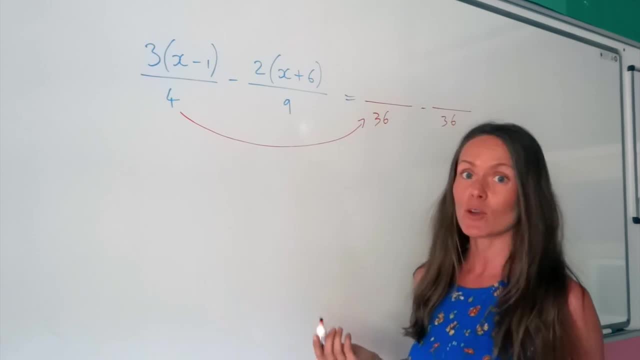 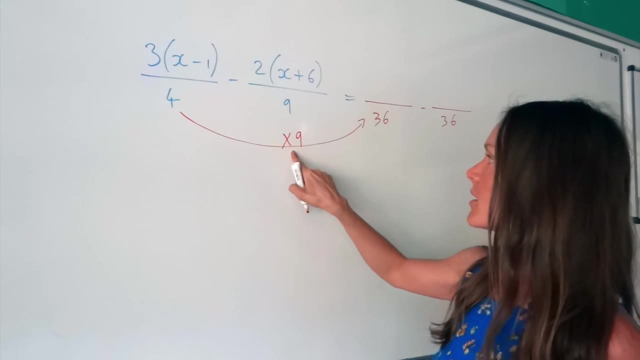 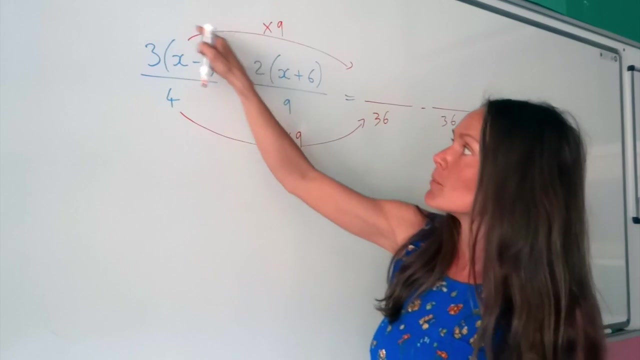 we need to change the numerators as well to find the equivalent fractions. So to change 4 to 36, I have to multiply that number by 9.. So I do the same with the numerator And I multiply this numerator by 9.. Well, when I multiply this by 9, I only need to multiply. 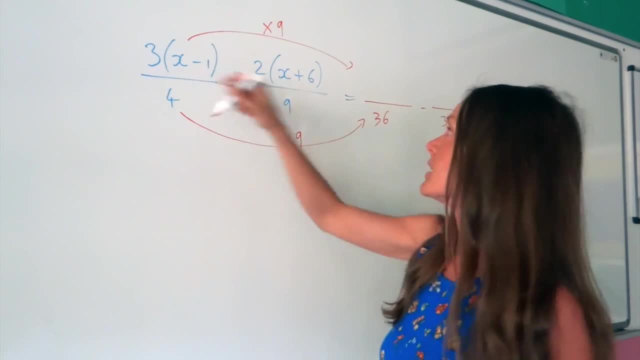 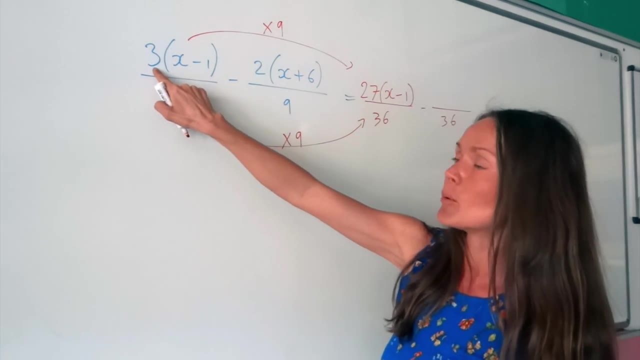 this number here by 9.. So 3 times 9. 9 is 27.. And this bracket? I can just leave that there for the moment. Okay, so multiplying this number by 9 is the same thing as multiplying this whole numerator by 9. And I'm going to. 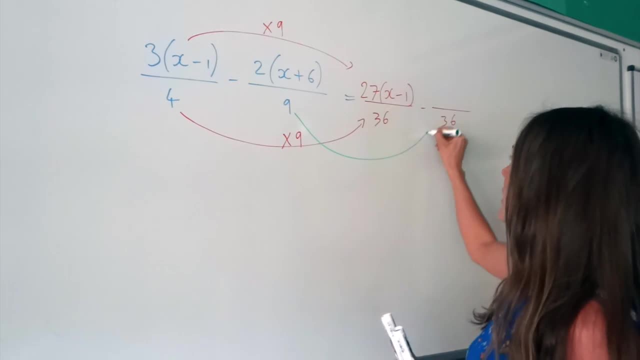 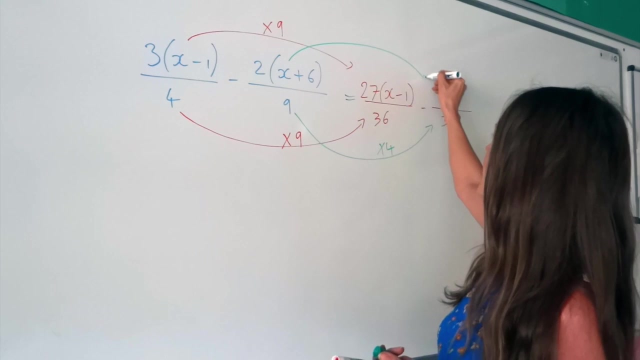 do exactly the same thing with the second fraction, except this time: to get from 9 to 36, we must multiply by 4.. So I'm going to do the same with this numerator And I'm going to multiply by 4.. So, just like before, you only need to multiply this number by 9.. 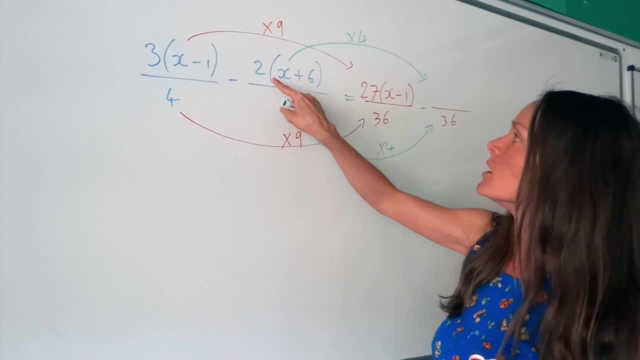 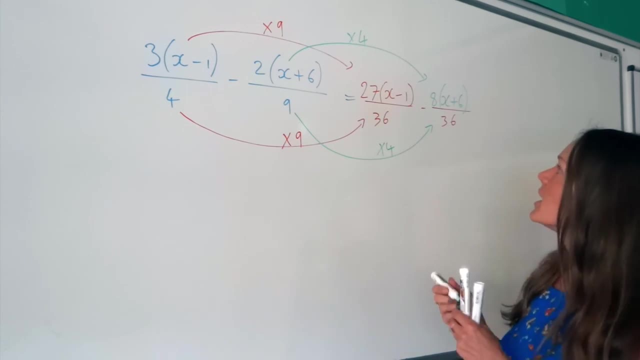 And I'm going to do the same with this numerator by 4.. It's the same thing as multiplying the whole thing by 4.. So 2 multiplied by 4 is 8. And the bracket just stays the same for the moment. Now I've got my common denominators here, So I can put them in one fraction. I. 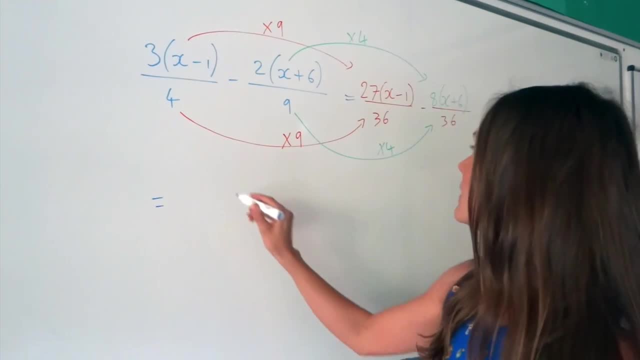 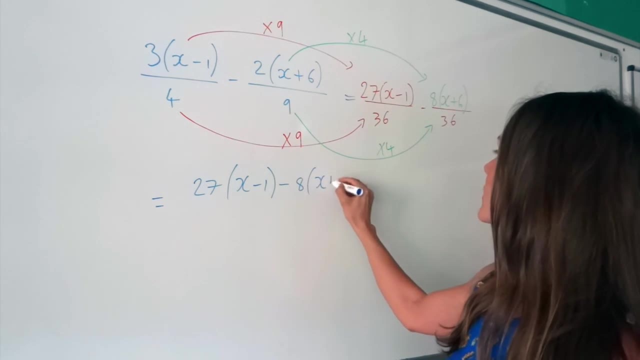 can start subtracting, So I'm going to continue just underneath. So I've got 27 brackets x minus 1. And then I've got minus 8 brackets x plus 6. Don't forget, you're subtracting these fractions. 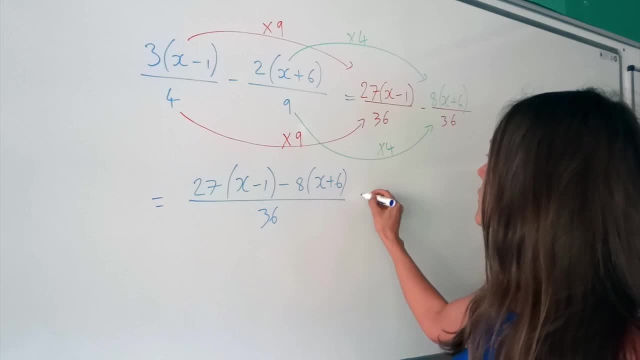 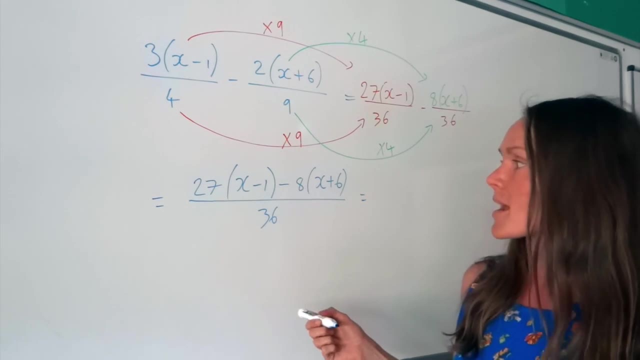 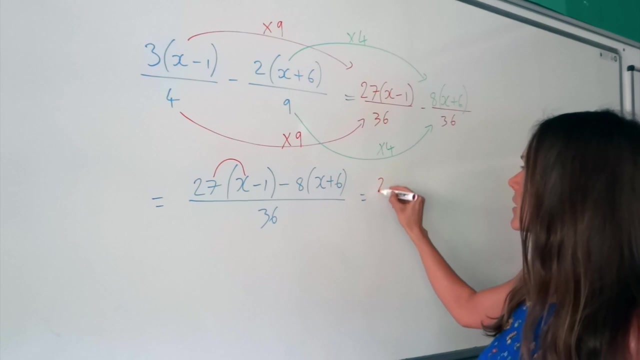 And the denominator is 36.. So we can't leave it like this. We need to get rid of these brackets. We need to multiply the brackets and then simplify. So let's multiply out to start with. So remember, brackets mean multiply. So you're doing 27 multiplied by x, which 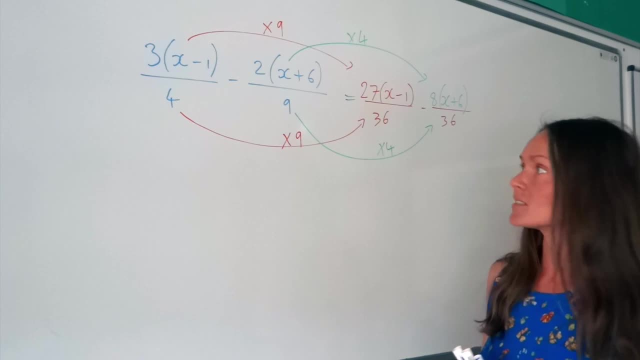 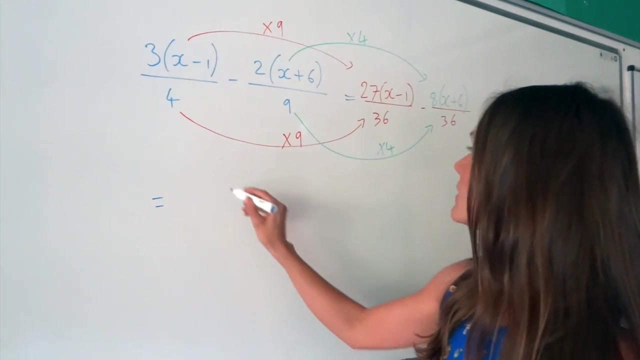 for the moment. Now I've got my common denominators here So I can put them in one fraction. I can start subtracting, So I'm going to continue just underneath. So I've got 27 brackets x minus 1.. 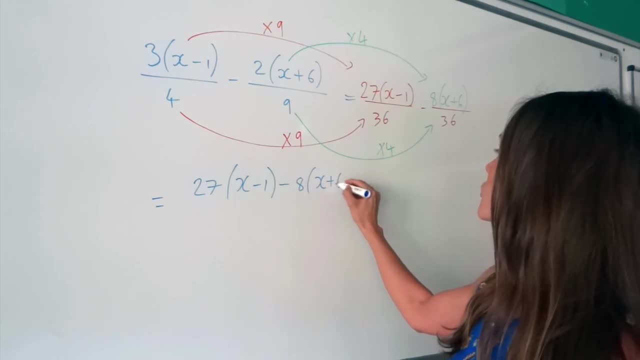 And then I've got my denominator. So I've got 27 brackets x minus 1.. And then I've got my denominator, minus 8 brackets x plus 6.. Don't forget: you're subtracting these fractions And the denominator is 36.. So we can't leave it like this. We need to get rid of these brackets. 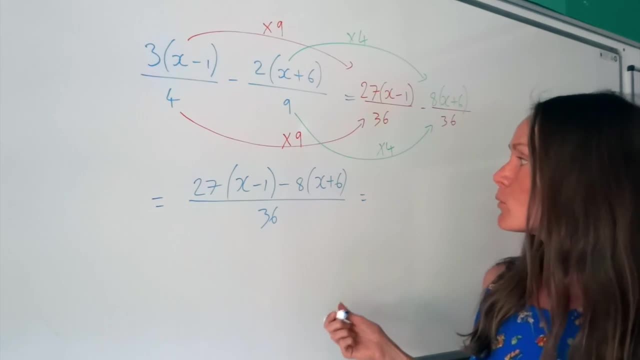 We need to multiply the brackets and then simplify. So let's multiply out to start with. So remember: brackets mean multiply. So you're doing 27 multiplied by x, which is 27x, And you're doing 27 multiplied by negative 1, which is negative 27.. 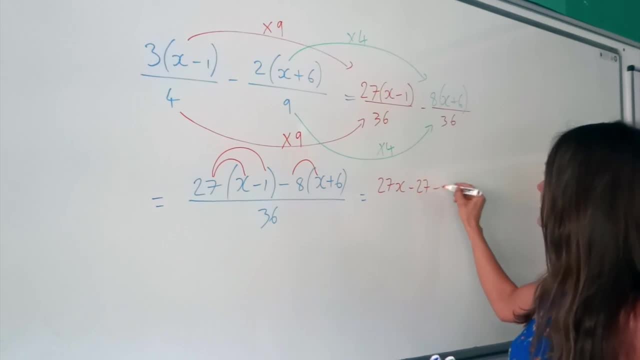 Then you've got negative 8 multiplied by x, which is negative 8x, And finally negative 8 multiplied by 6, which is negative 48. Now, remember, the denominator is still 36.. And now we can simplify those terms. 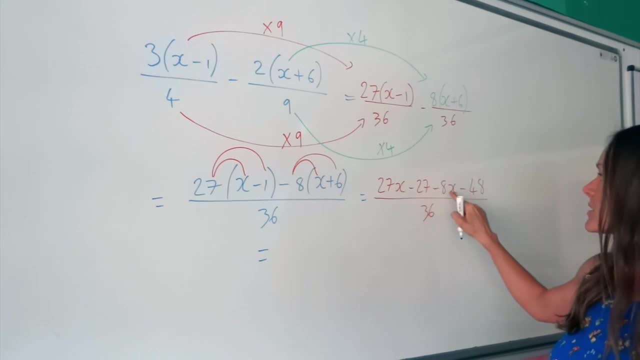 So we've got x terms here. We've got 27x minus 8x, which is 19x, And we can add the numbers together too, So we've got negative 27 plus negative 48, which is negative 75.. 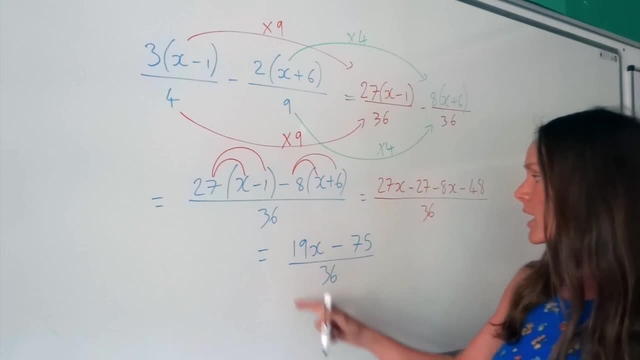 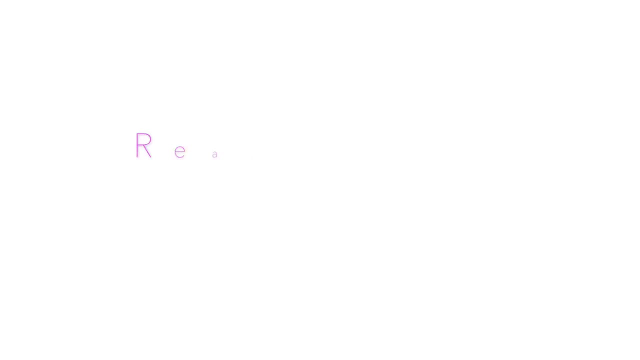 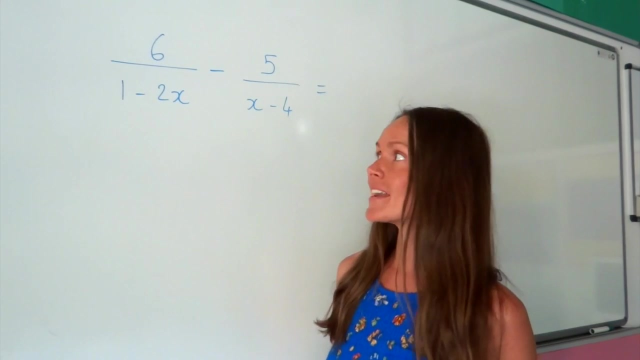 And again, the denominator stays the same. So we don't have a common factor. So I'm just going to leave this fraction as it is. I can't simplify it. OK and one more. OK, and now for the last example. 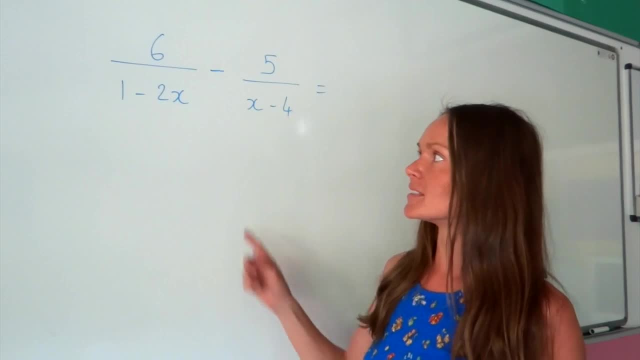 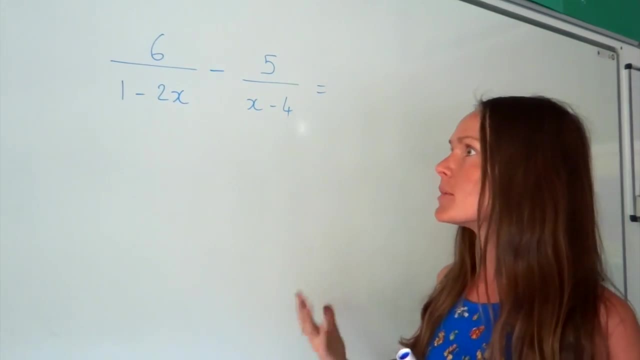 So this one looks a bit strange. It's strange because the denominators they're not just single numbers anymore, Now they're expressions, They're a mixture of numbers and letters, So it's a bit difficult to find multiples of these and finding the lowest common multiple. 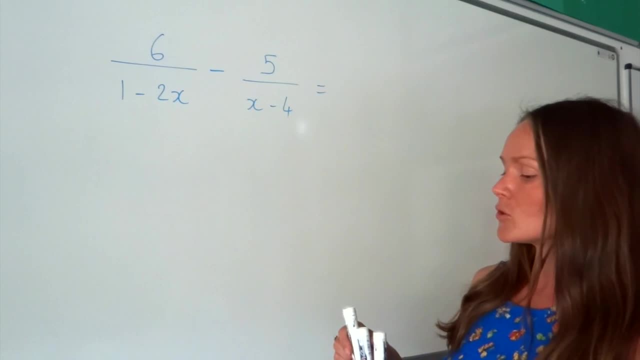 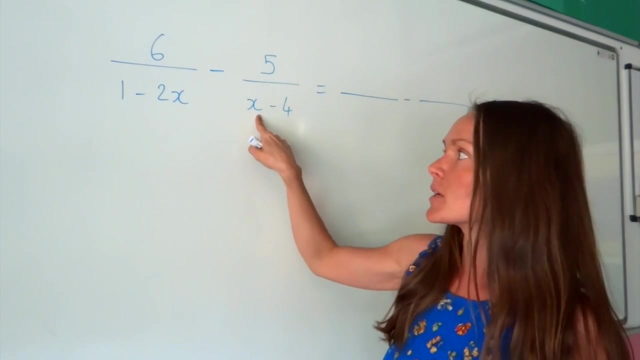 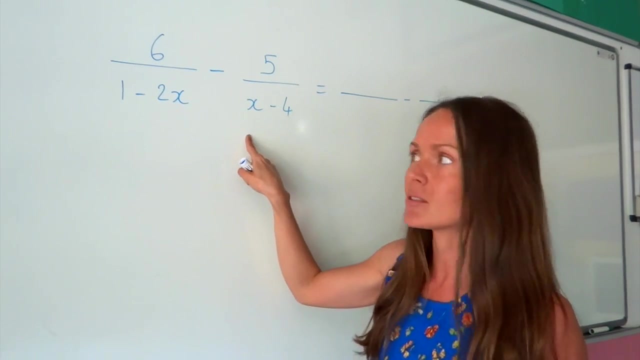 So when you get a question like this, all you have to do is to find the common denominator. multiply these two denominators together, Because if you multiply those two numbers together, that answer has to be a multiple of those two. OK, so that's going to be the new denominator in our equivalent fractions. 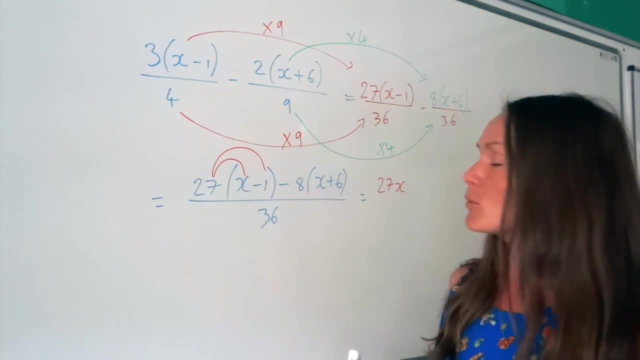 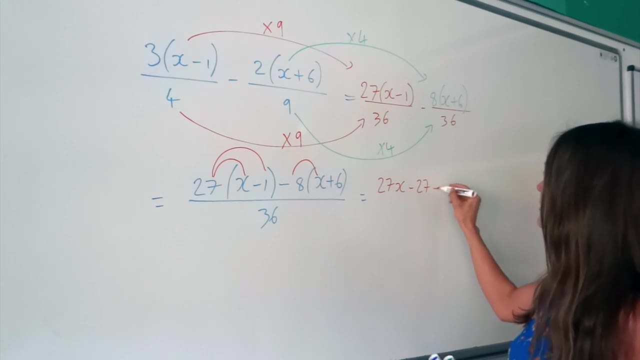 is 27x, And you're doing 27 multiplied by negative 1, which is negative 27.. Then you've got negative 8 multiplied by x, which is negative 8x, And finally negative 8 multiplied by 6, which is negative 48.. Now remember the denominator. 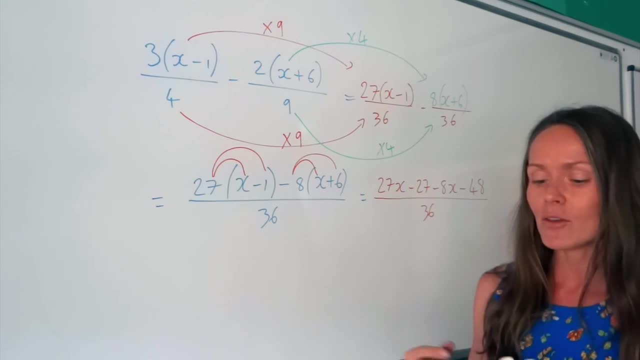 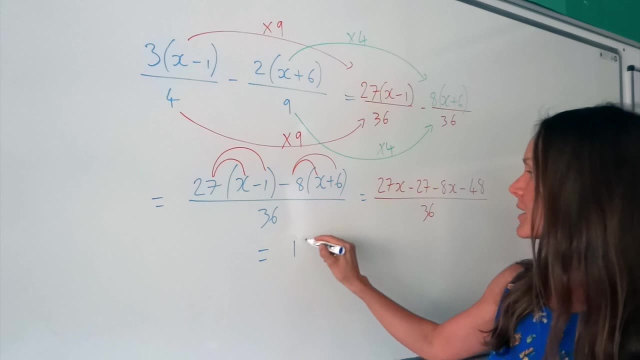 is still 36.. And now we can simplify those terms, So we've got x terms here. We've got 27x minus 8x, which is 19x, And we can add the numbers together too, So we've got negative. 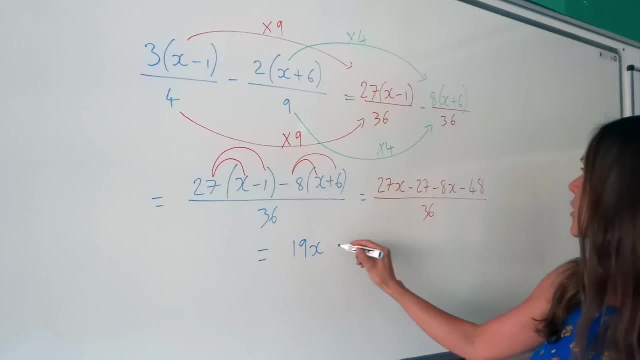 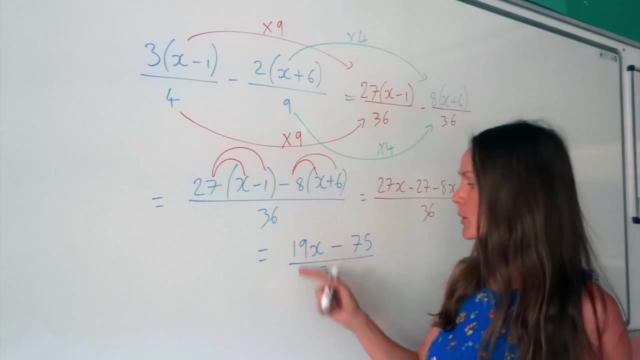 27 plus negative 48,, which is negative 75.. And again the denominator is still 36.. And the denominator stays the same. So we don't have a con factor. So I'm just going to leave this fraction as it is. I can't simplify it. 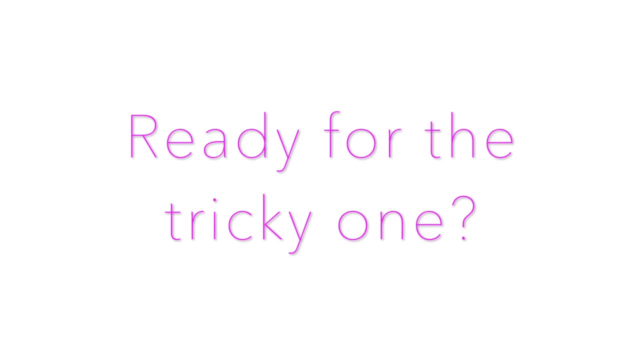 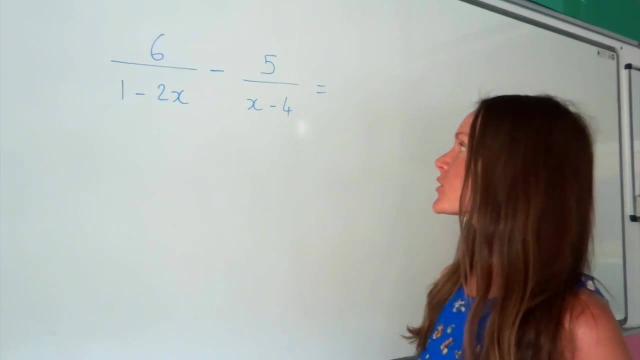 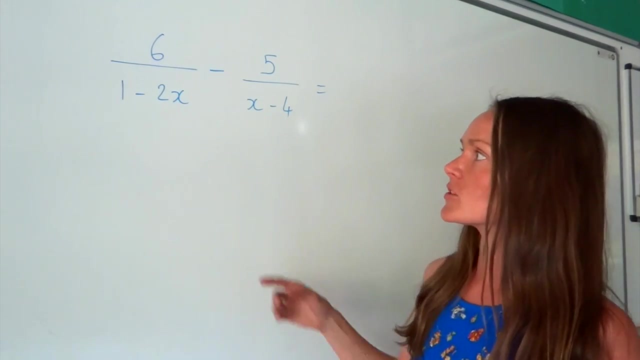 OK, and one more OK. and now for the last example. So this one looks a bit strange because the denominators they're not just single numbers anymore, Now they're expressions, They're a mixture of numbers and letters. So it's a bit difficult to find more than one denominator. So we're 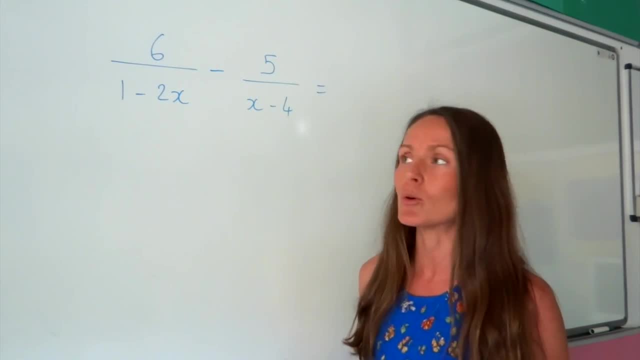 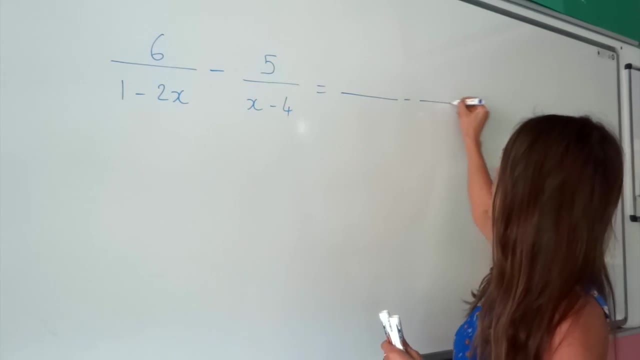 going to find multiples of these and finding the lowest common multiple. So when you get a question like this, all you have to do is to find the common denominator, multiply these two denominators together, Because if you multiply those two numbers together, that 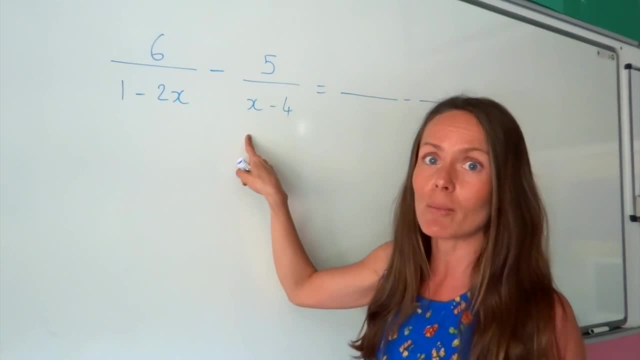 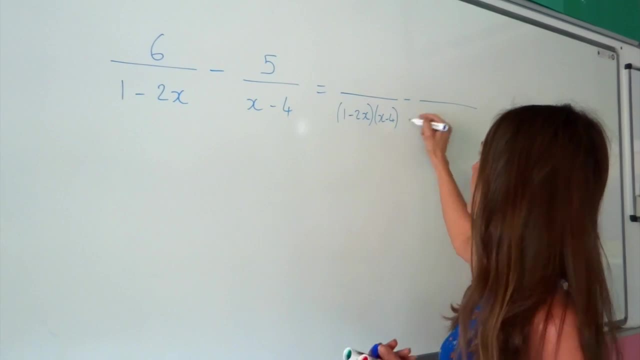 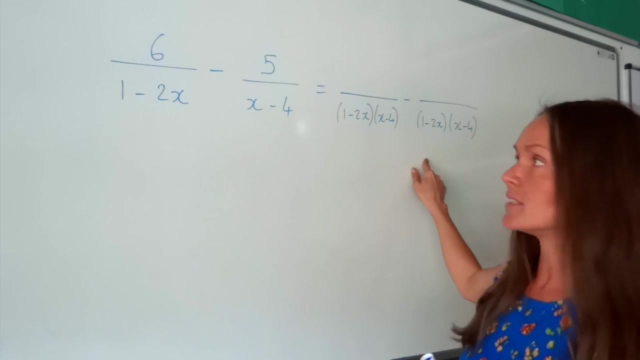 answer has to be a multiple of those two denominators. OK, so that's going to be the new denominator in our equivalent fractions And I'm going to leave those in brackets. I'm not going to expand the brackets. OK, so we found the common denominators. Now we need to find the equivalent fractions. 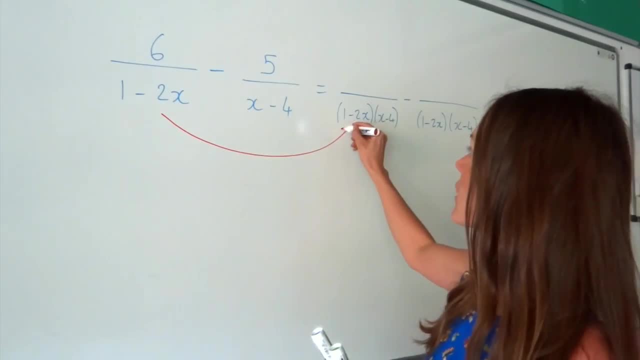 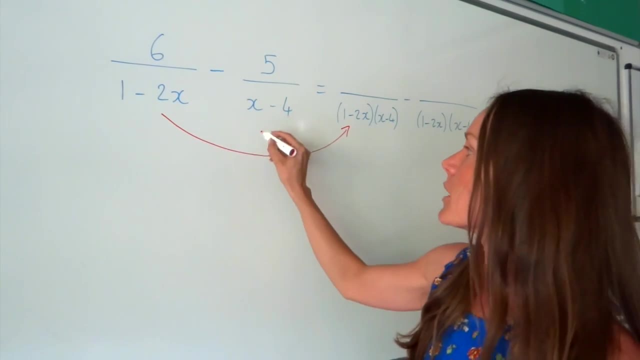 So we need to find the numerator part So to get from the first fraction to over here. well notice how we've now got the x minus 4 underneath. So we multiply by x minus 4.. Don't forget you need to do the same with the top. So we're multiplying that number. 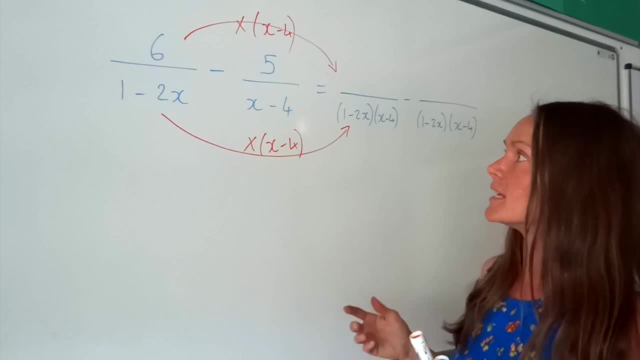 6 by x minus 4 as well. So really you're just multiplying the top and bottom of the fraction with x minus 4.. OK, so let's work that out. 6 multiplied by x is 6x And 6 multiplied. 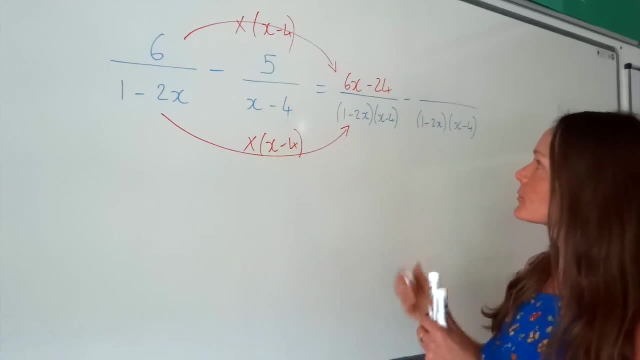 by negative 4 is negative 24.. Now for the second fraction. Again, the denominator has changed. We've got 1 minus 2x underneath. that wasn't there before. So we're multiplying by 1 minus 2x. So, if you like, you're just multiplying. 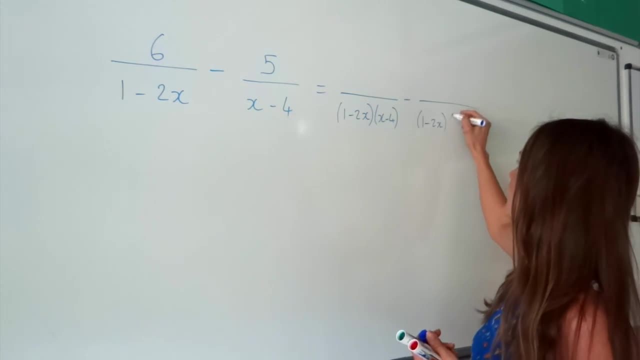 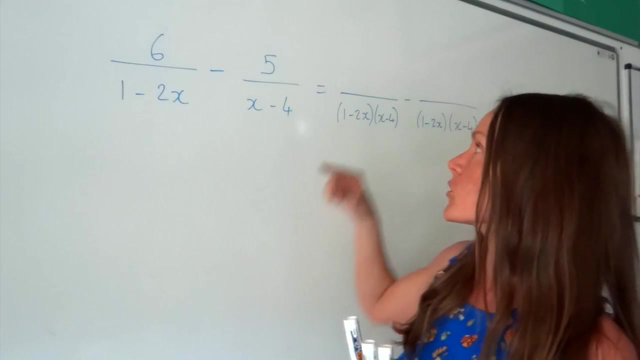 And I'm going to leave those in brackets. I'm not going to expand the brackets. OK, so we found the common denominators. Now we need to find the equivalent fractions. So we need to find the numerator part. So to get from the first fraction to over here, 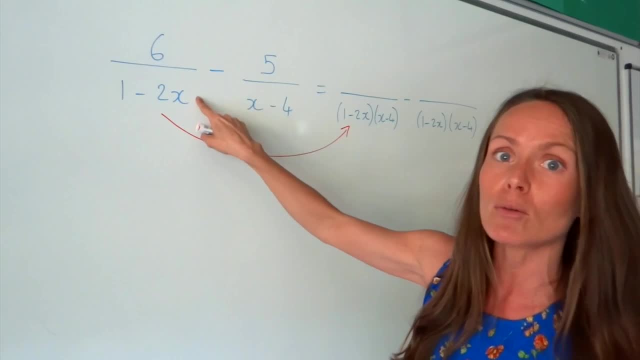 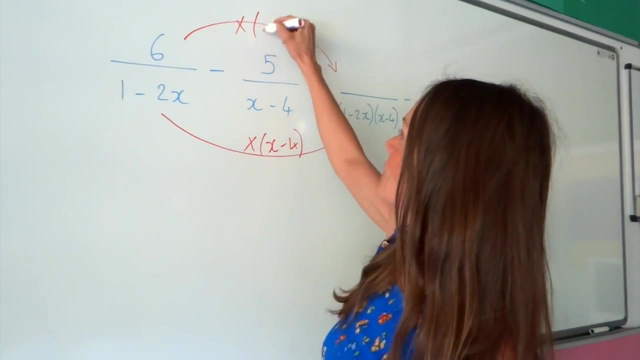 well notice how we've now got the x minus 4 underneath. So we multiply by x minus 4.. Don't forget, Don't forget, Don't forget. You need to do the same with the top. So we're multiplying that number 6 by x minus 4 as well. 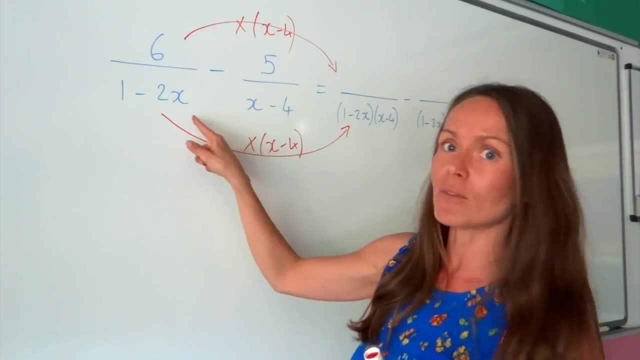 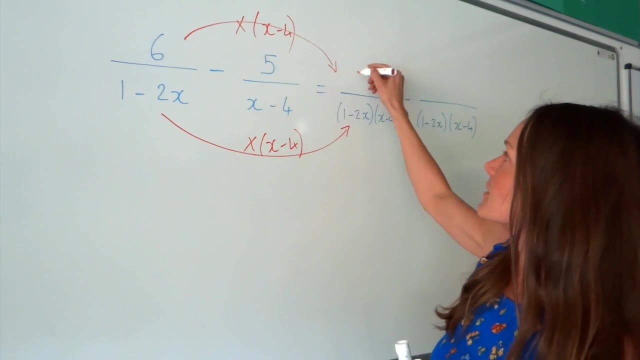 So really, you're just multiplying the top and bottom of this fraction with x minus 4.. OK, so let's work that out: 6 multiplied by x is 6x, And 6 multiplied by negative 4 is negative 24.. 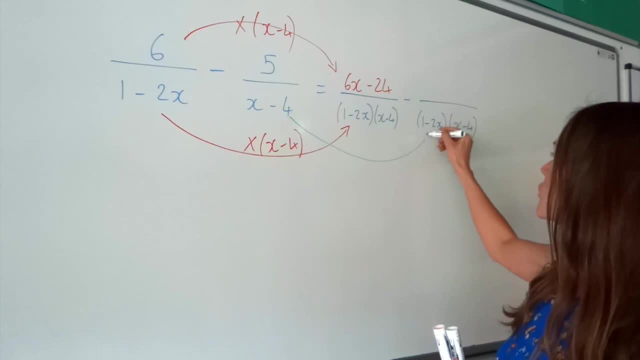 Now for the second fraction. Again, the denominator has changed. We've got 1 minus. We've got 1 minus 2x underneath. that wasn't there before. So we're multiplying by 1 minus 2x. So, if you like, you're just multiplying the top and bottom of this fraction by this denominator here. 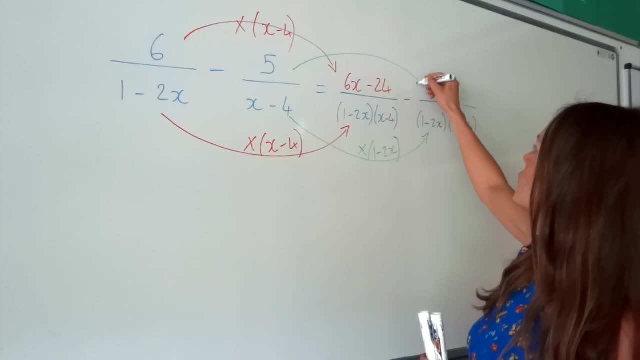 So 1 minus 2x. So we need to do the same with the numerator. So again, we're timesing by 1 minus 2x. Remember, it's always the same thing for the top and the bottom. So I'm going to work that out. 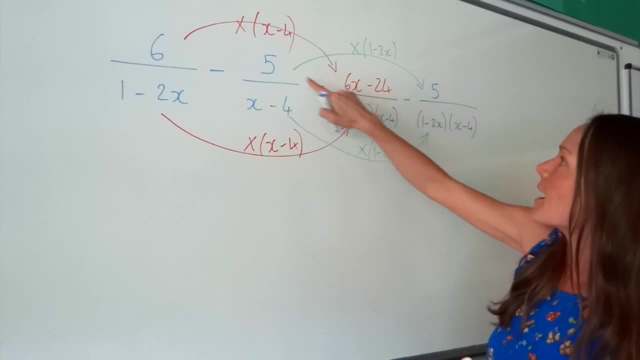 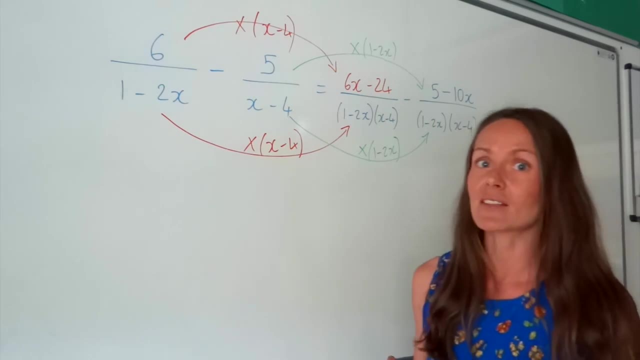 5 multiplied by 1 is just, It's just 5.. And 5 multiplied by negative 2x is negative 10x. Now watch out for these subtract algebraic fractions, Because lots of people make an error and they forget to subtract everything. 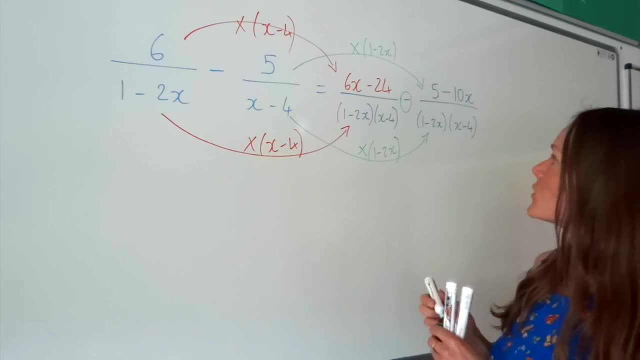 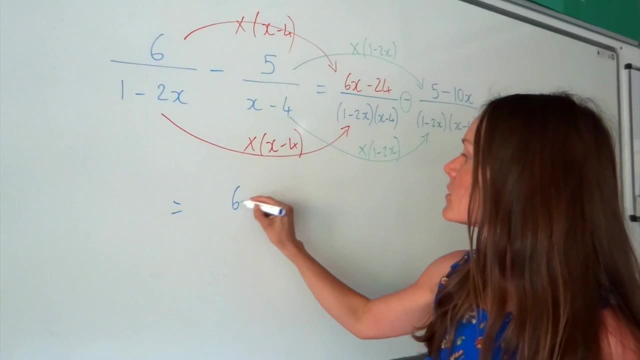 OK, so do please watch out for that minus. So down here I'm going to continue the question. I'm going to start putting them all on one fraction. So I've got 6x minus 24 for the first numerator part. 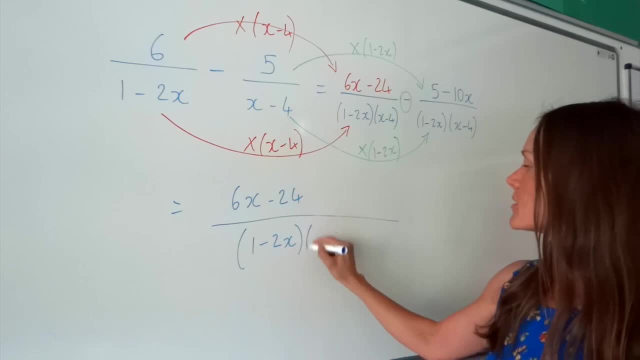 The denominator. remember that stays the same. It hasn't changed. But for the next part, I'm going to leave my minus sign in And I'm going to put this numerator into brackets, Because that negative sign is going to affect all of this on the top. 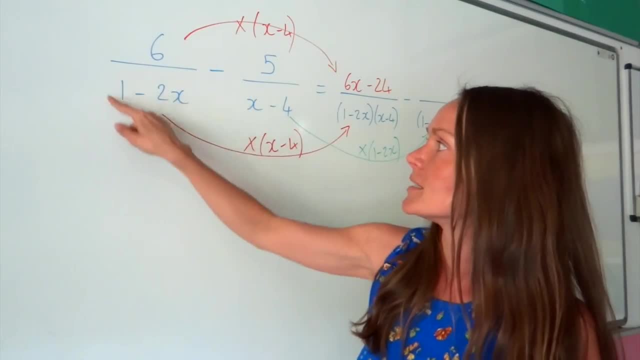 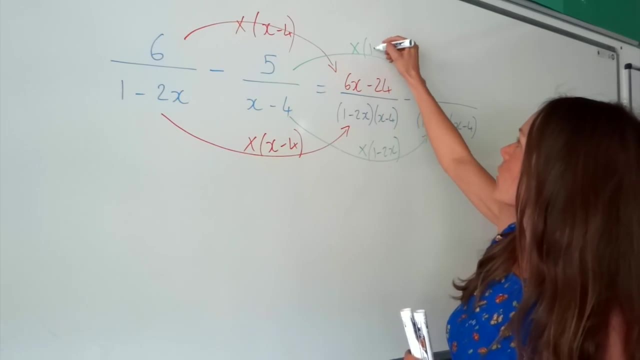 the top and bottom of this fraction by this denominator here. so 1 minus 2x. So we need to do the same with the numerator. So again, we're timesing by 1 minus 2x. remember It's always the same thing for the top and the bottom. 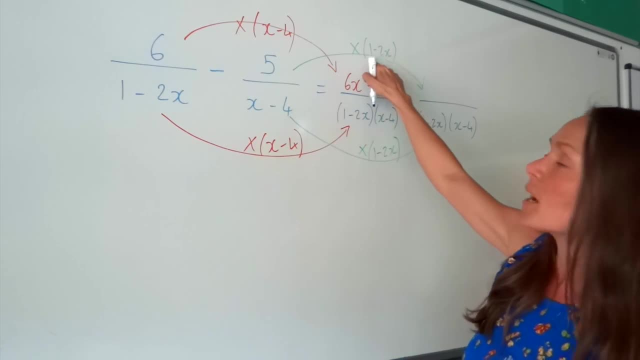 So I'm going to work that out: 5 multiplied by 1 is just 5, and 5 multiplied by negative 2x is negative 10x. Now watch out for these subtract algebraic fractions, because lots of people make an error and they forget to subtract everything. 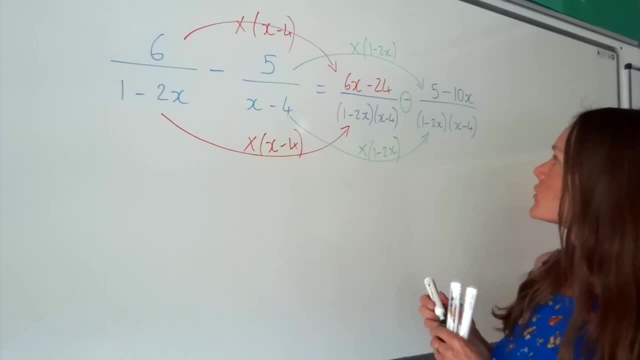 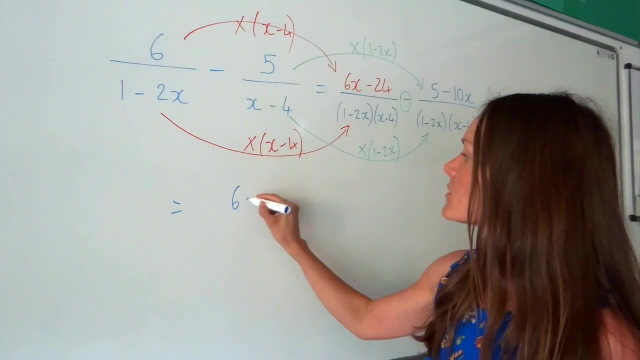 Okay, So do please watch out for that minus. So down here I'm going to continue the question. I'm going to start putting them all on one fraction. So I've got 6x minus 24 for the first numerator part. 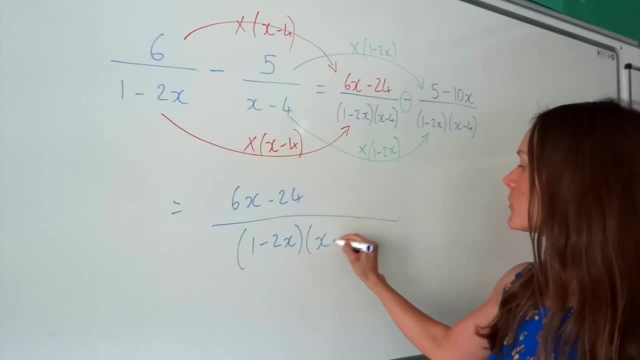 The denominator- remember that- stays the same, hasn't changed. But 4x minus 24 is negative 10x. For the next part, I'm going to leave my minus sign in and I'm going to put this numerator into brackets. 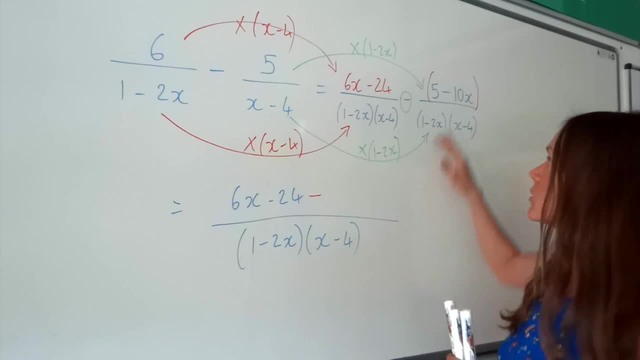 because that negative sign is going to affect all of this on the top, not just the first part, but all of it. So if I put that in brackets, you can see that not only are we going to minus 5, but here we've got a double minus which will actually turn into a plus. 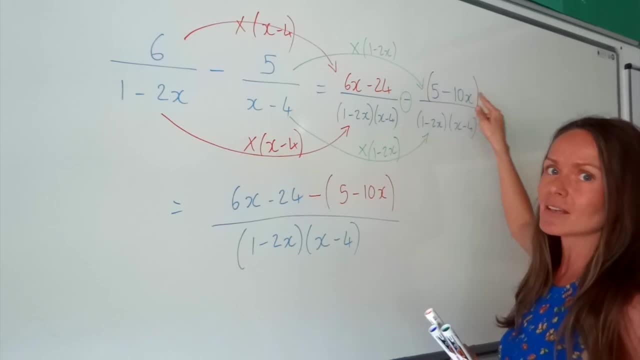 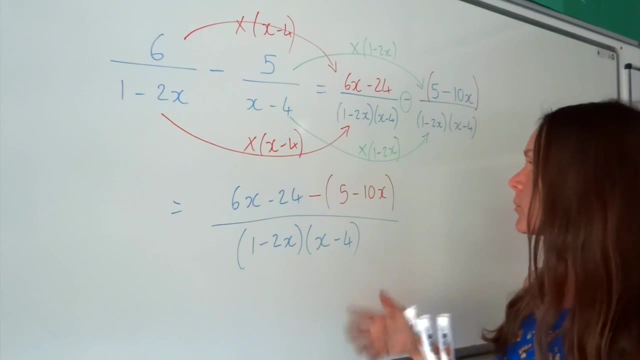 So whenever, So whenever you're subtracting, leave that numerator in brackets, so to remind yourself that that negative will affect everything inside those brackets. So now I'm going to work it out. So I've got 6x minus 24 stays the same for the moment. 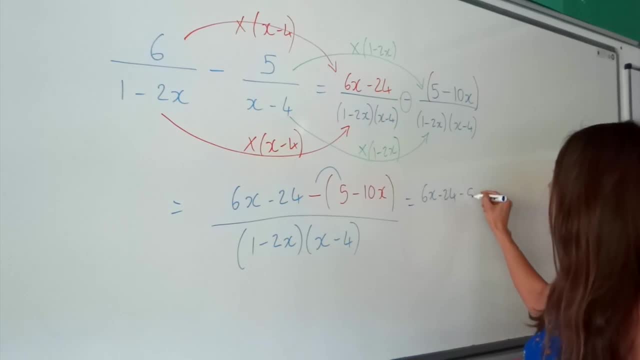 Here I've got minus 5,, okay, And then I've got a minus times a minus, which is a plus. And remember you're just, This is like an invisible 1 here. So you're doing minus 1.. So you're doing minus 1 times minus 10x, which is just plus 10x. 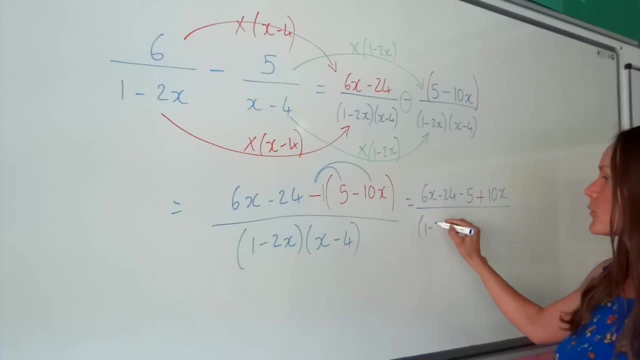 And remember the denominator. we're going to leave factorised like that. We don't need to expand the brackets, So keep going. It's a long question, but we're nearly there. Simplify the numerator. We've got x terms here that we can add together. 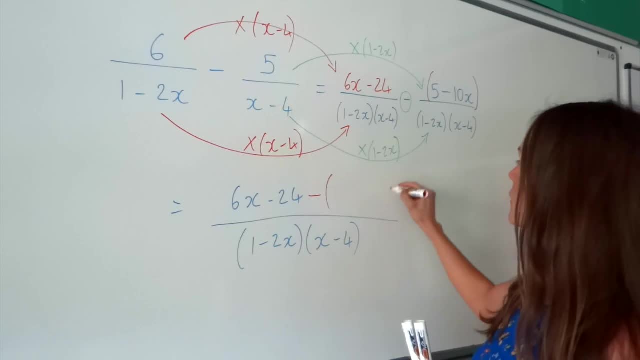 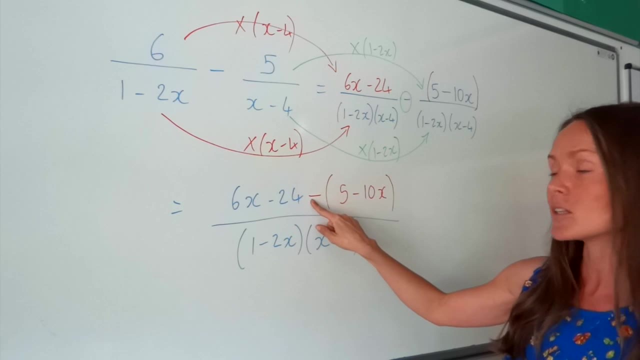 Not just the first part, but all of it. So if I put that in brackets, you can see. You can see that not only are we going to minus 5, but here we've got a double minus which will actually turn into a plus. 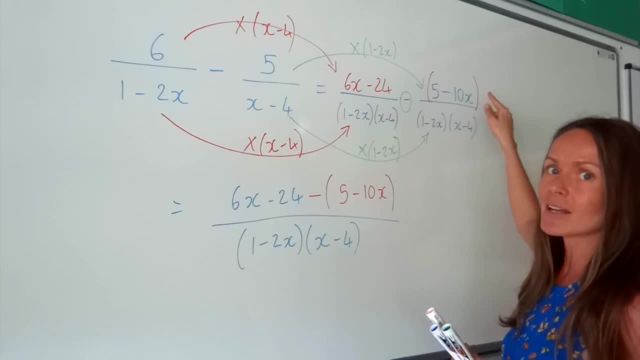 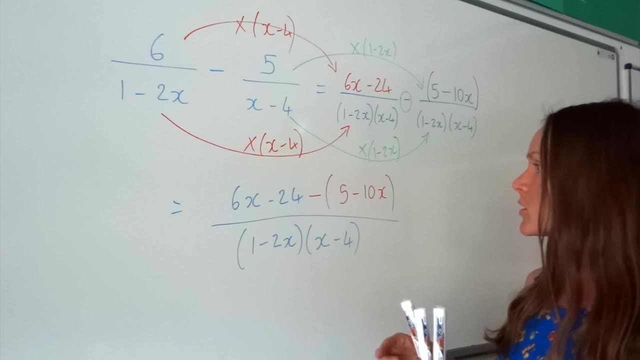 So whenever you're subtracting, leave that numerator in brackets, So to remind yourself that that negative will affect everything inside those brackets. So now I'm going to work it out. So I've got 6x minus 24. stays the same for the moment. 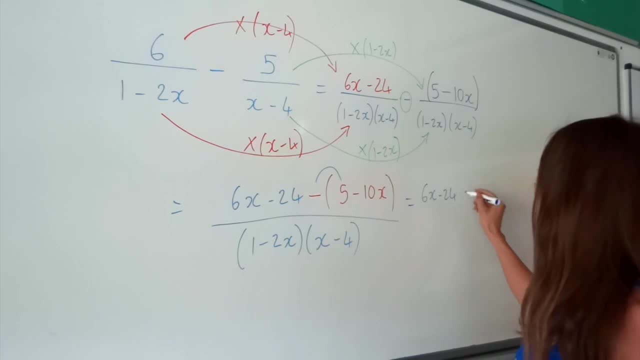 Here I've got minus 5.. OK, and then I've got a minus times a minus, which is a plus, And remember, this is like an invisible 1 here. So you're doing minus 1 times minus 10x, which is just plus 10x. 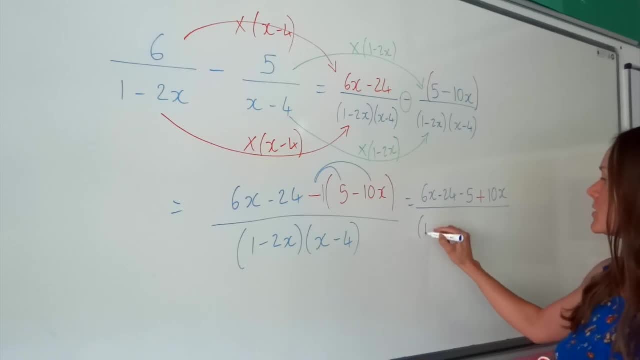 And remember the denominator. we're going to leave factorised like that. We don't need to expand the brackets, So keep going. It's a long question, but we're nearly there. Simplify the numerator. We've got x terms here that we can add together. 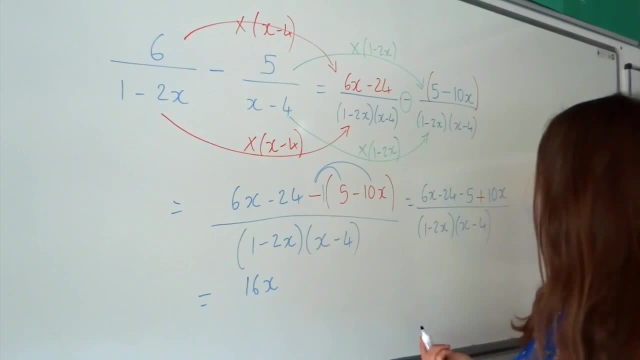 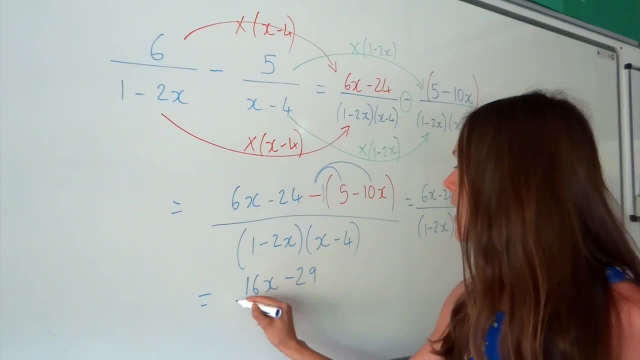 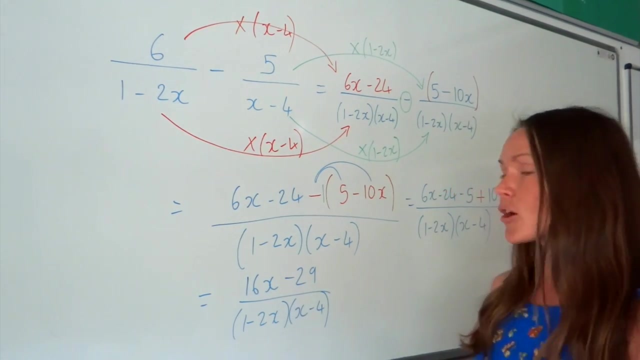 So 6x plus 10x is 16x. Then we can subtract these numbers, So negative 24 minus another 5 is minus 29.. And the denominator I'm going to leave like that. OK, so that was long, but we got there in the end. 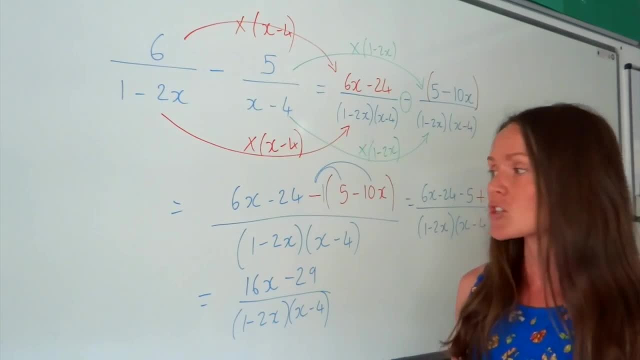 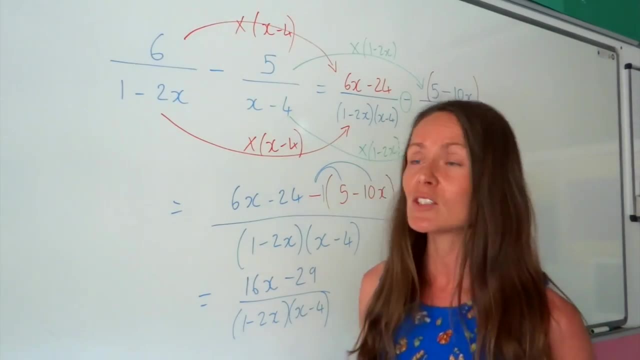 So watch out for those subtracting algebraic fractions, because lots of people get caught out when they're subtracting the second part. Hopefully, with more practice, you won't need to draw lines everywhere like I've been doing in my examples, And I'll have some more videos coming up soon. 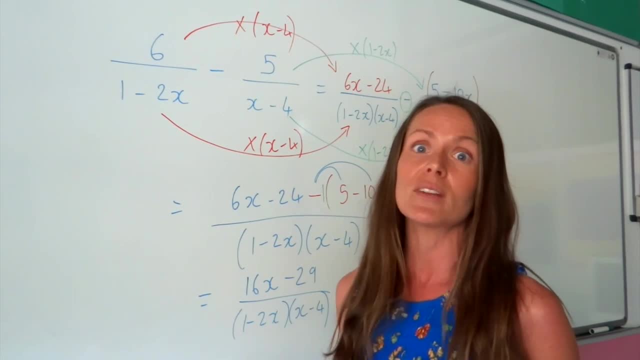 for simplifying algebraic fractions and solving equations with algebraic fractions. So OK, bye-bye for now. 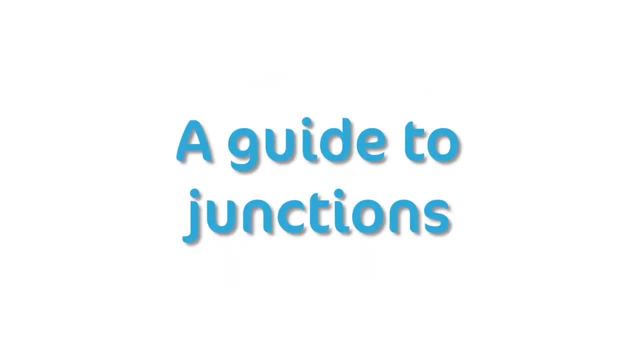 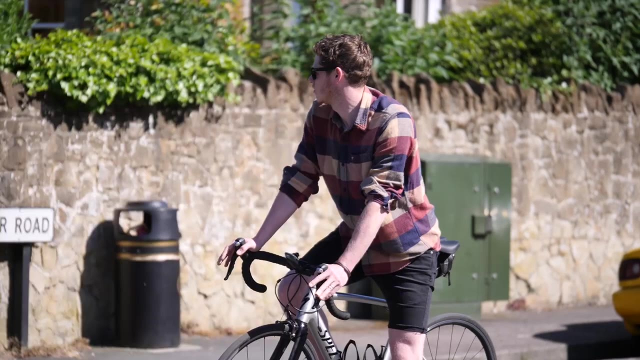 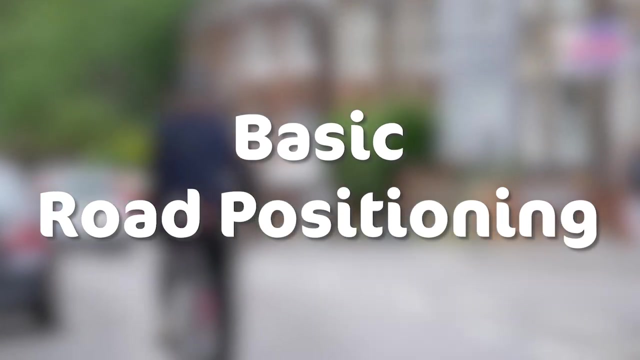 More than 70% of collisions involving a bike happen at or near a junction, so we're going to take you through the most common junctions and how to manoeuvre around them. Basic road positioning. While cycling, your basic road position should be at least an.